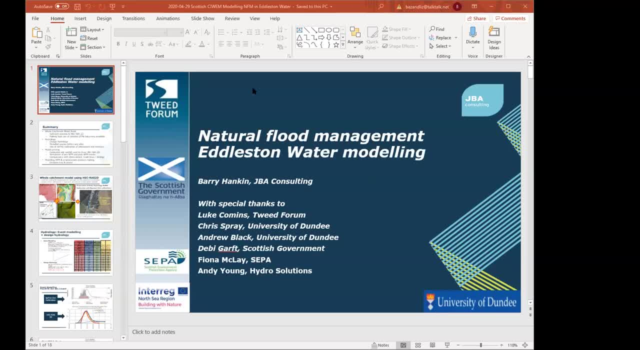 He's also a visiting lecturer at LEC, Lancaster University, working on the QNFM project, investigating the effectiveness of NFM. This evening he is going to be speaking on his natural flood management work on the Eddleston water and would like to acknowledge key partners and others who have worked on the Eddleston water project. 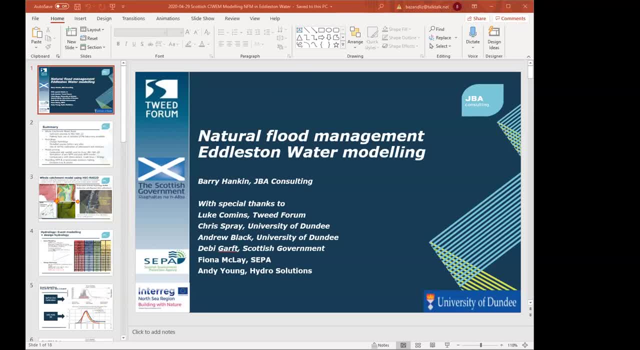 Thank you, Barry Carlin. Thank you, Please post your questions via the message feature on Zoom. We will aim to work through them as many as possible. Thank you Over to you, Barry. Barry Carlin, Great, thank you very much, Alice. 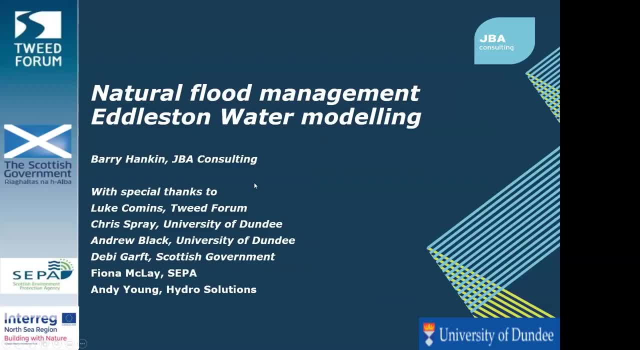 I'm just trying to start my slideshow. There you go, There we go. it should be in presenter mode now, and thanks very much for that introduction. Yeah, of course I'd like to thank the people listed, without whom the modelling work wouldn't. 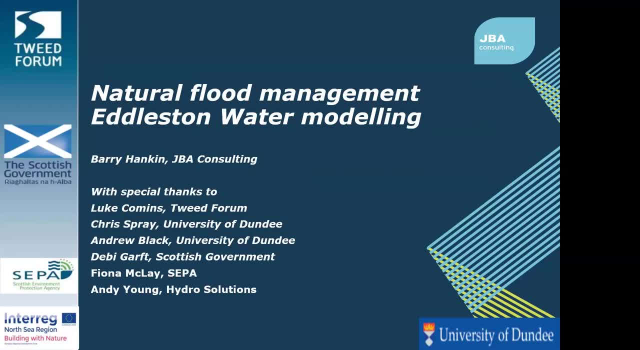 be possible without the hard years of, I guess, obtaining grants and installing NFM: installing monitoring in one of the most foremost instrumented catchments in Scotland, with 14 hydrometric sites and an awful lot of NFM installed between 2012 and 2015,, including native tree. 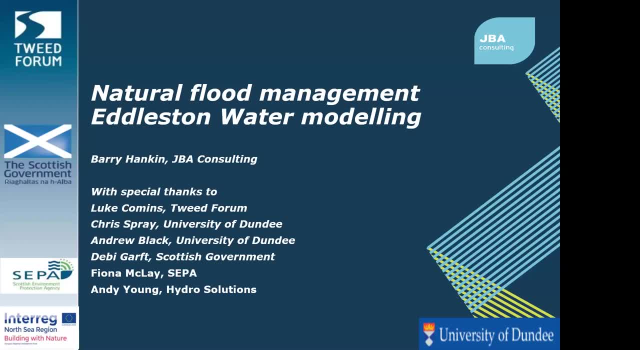 planting engineered log jams, re-meandering ponds and so on. Now the aim of this work was to see if we could represent NFM and understand the whole system response, and whether such a model could be used to represent NFM effectively. 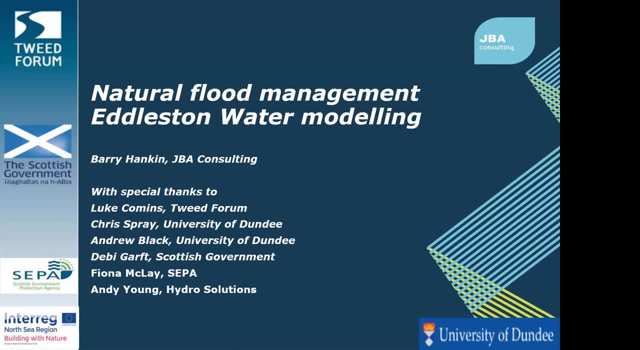 So we want to demonstrate how NFM can be appraised alongside other traditional risk reduction methods. So this project was to see how far we could push whole catchment modelling, whole system modelling, to understand the responses and how we could represent NFM. 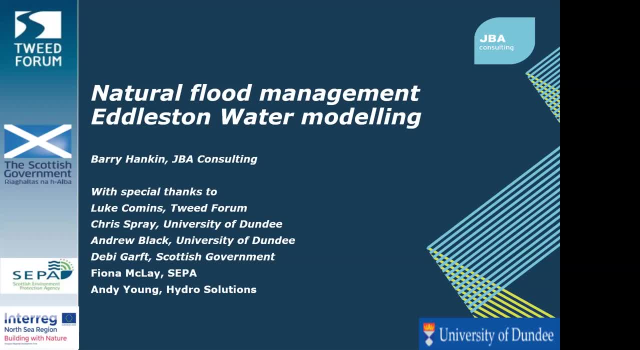 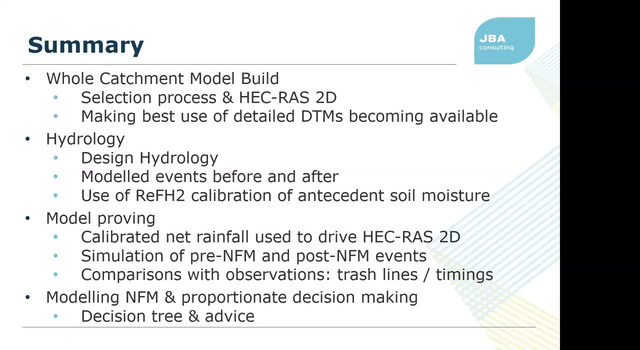 One of the issues, of course, is just how do you represent NFM? And there are three main issues And there are three major NERC UK studies ongoing at the moment and I'll refer to those as we go along. So in summary of my talk I'm going to cover the whole catchment model build and how we 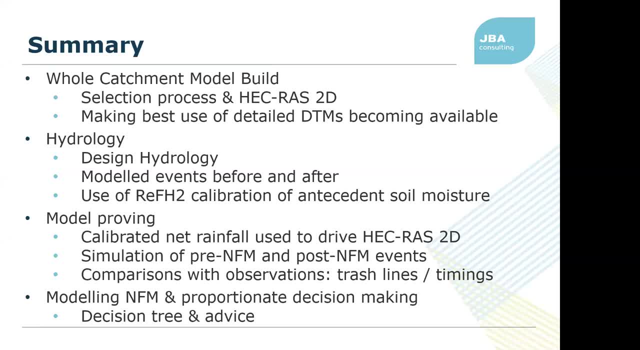 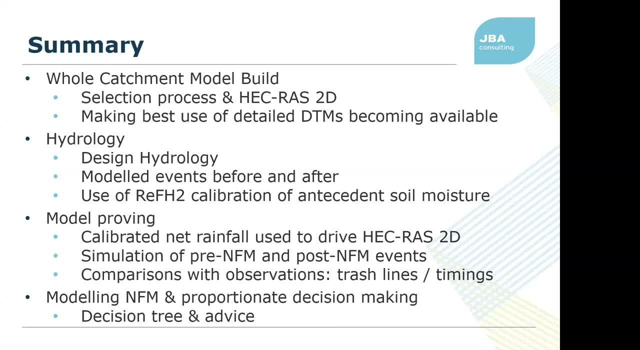 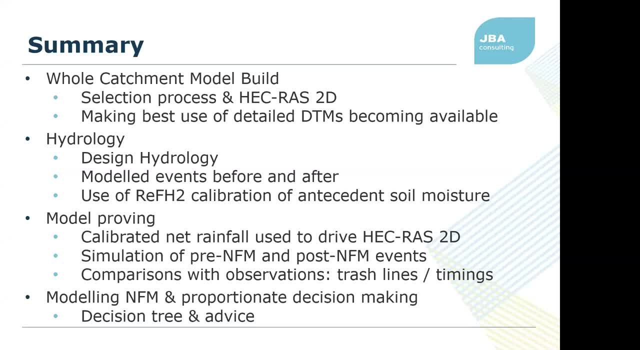 has been a very engaged process and we want the model to have longevity and we want to be able to share it with people, And HECRAS-2D is one of those models that doesn't need a license from the US Army. 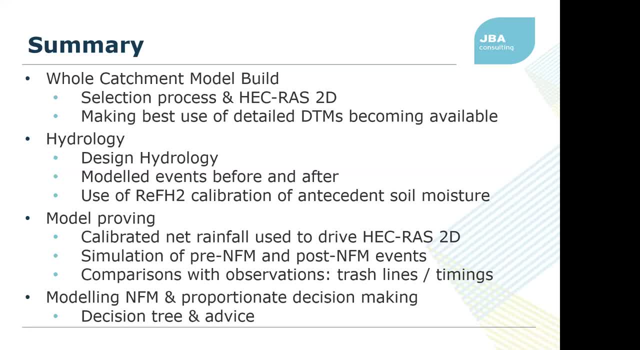 Corps of Engineers, making it very flexible. I'm going to cover those sort of aspects. I will not be talking about the HECRAS-2D model aspects and i'm going to get stuck into some of the whole catchment calibration that we've done. 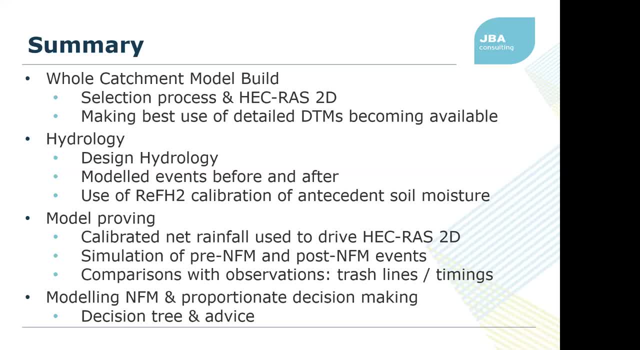 using that framework, i'm going to kind of skip over more of the sort of decision processes that went into that um, but don't be afraid to contact me out with this because there's a lot of different modeling platforms that could be used. um, and i'm going to cover the hydrology. so for this study we we looked at design hydrology and 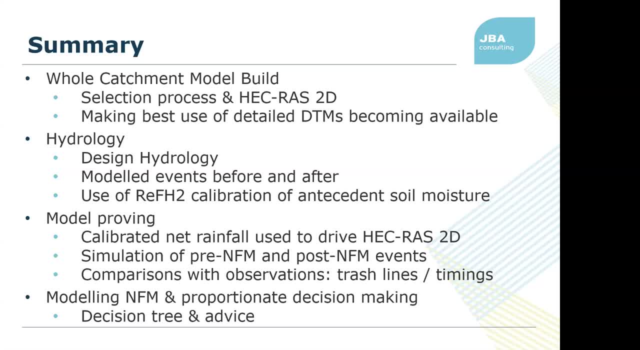 event hydrology- uh. we modeled events before and after uh using making use of the distributed monitoring data from the different gauges that the university of dundee and others have been generating data from since about 2012- 2011.. and um, we um sort of covered statistical methods and ref h2 calibration methods. 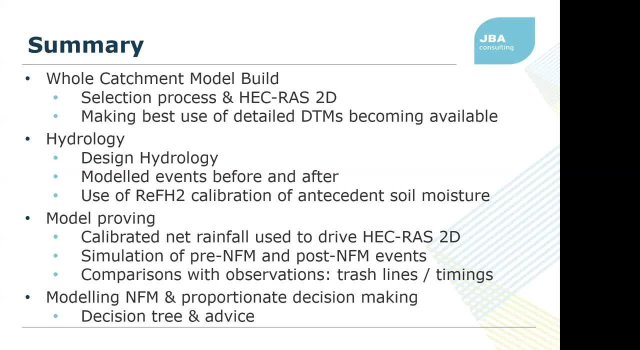 so that we could be sure that we were getting the initial antecedent soil moisture right and modeling some real events. there haven't been a whole load of large events, apart from this year, which is typical. so after we calibrated the post nfm scenario, there have of course been some. 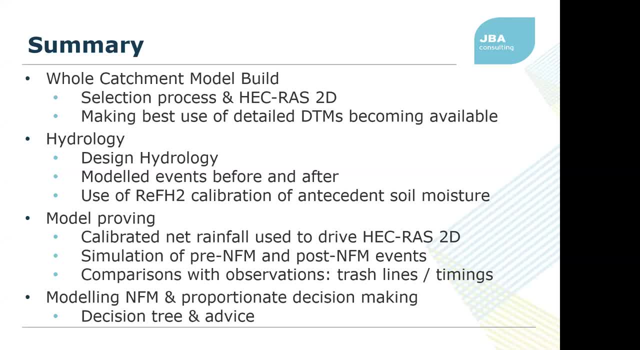 larger events like stormkira and dennis in 2020, um, but more of that in a bit um with. so what we've done is we've um, we have um done um a degree of model proving, using, uh the event data that we have. we have some uh trash line surveys, uh for a slightly peculiar event in june 2012, and we've made comparisons with observations. 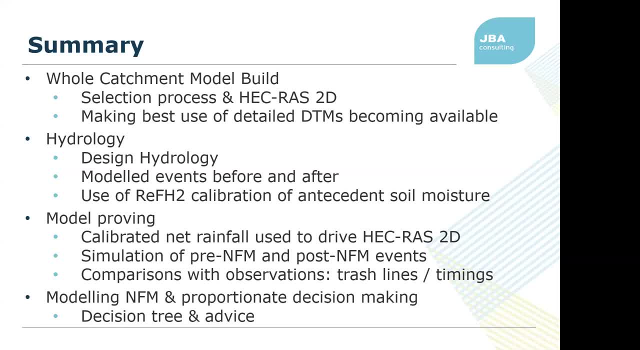 and tried to sort of show, uh, that the model represents the system well. but of course, this could all be done in an uncertainty framework and we are at this moment, uh, running multiple simulations to try and understand that the quantum of uncertainty, um. so um, we'll talk about also how. 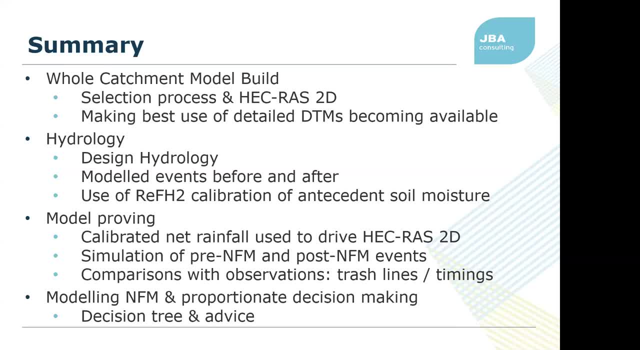 other projects can learn from this one, and one of the outputs is a user guide with the model. so there'll be the digital deliverables in terms of that cross 2d model and all the data, and that comes with a user guide and a sort of decision tree process for understanding what level of modeling might. 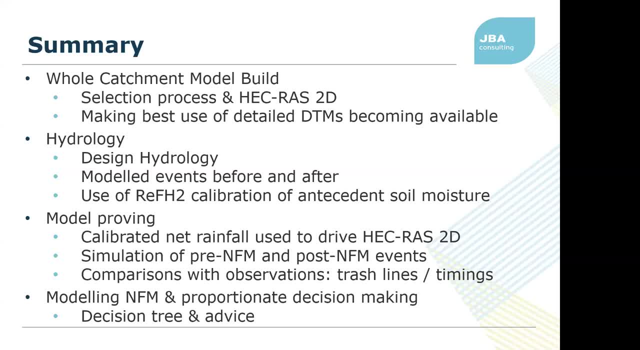 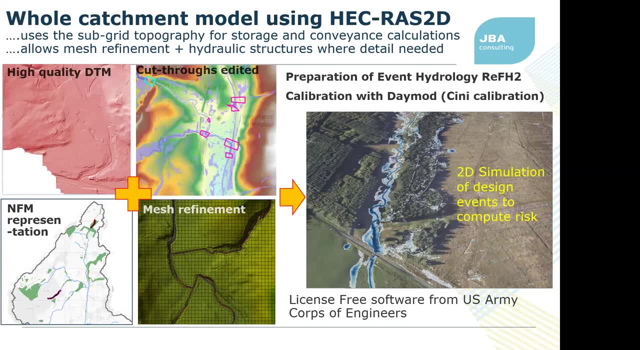 be needed to appraise nfm in the mix when you're combining it with traditional risk reduction methods. so i'm getting straight into the detail. um, let's just sort of step back a little bit again and talk about the data set across two d. well, we want to be able to make use of these emerging data. 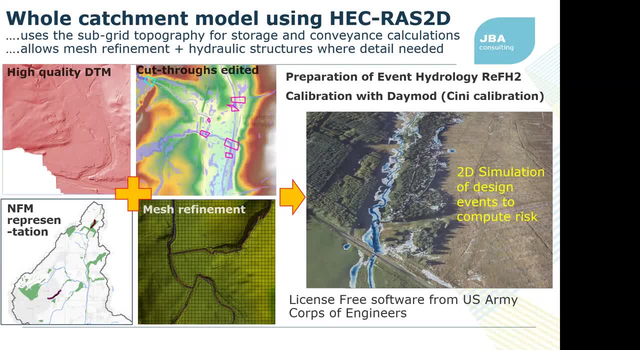 sets that have got high resolution topography. so when we've got lidar at half a meter for 70 kilometers squared catchment, that means we've got about um 290 million pixels um, and we've got an awful lot of detail there. and i suppose one of the questions is: well, how do we best make use of that? 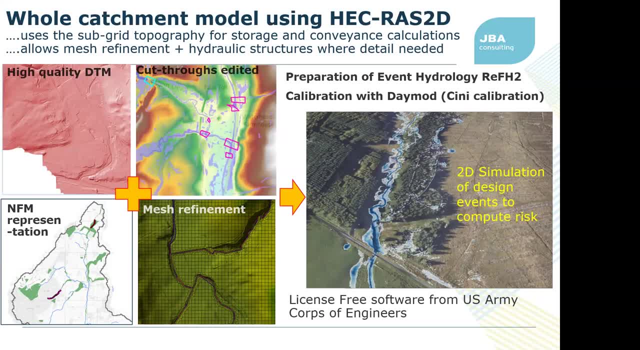 uh search. your cell size is quite difficult to model. we can just about do that. We used a similar number of cells in the model of the Eden catchment in the DEFRA flood modelling competition. but it does also take a long time to simulate, even on a. 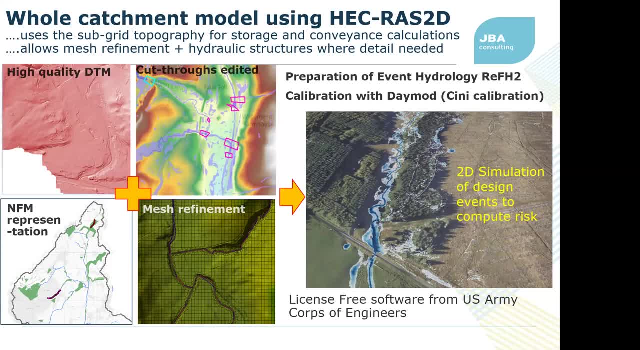 graphics processing card. So there are emerging techniques and HECRAS has sort of gone straight in there with version 5 to allow the subgrid topography to be represented in a course that has a mesh. So the way it does that is it builds hydraulic tables of the subgrid. so it has a look. 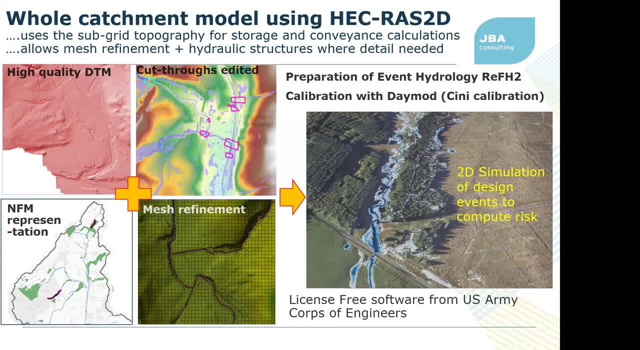 up between the level and the storage within that cell, all based on the half metre resolution DTM. And it does the same across the flow, across the faces. So we have conveyance tables against elevation as well. And if we move from the sort of pink inset diagram to the next one on the right, 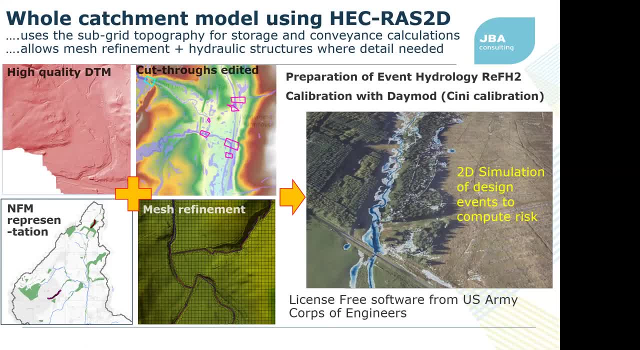 we have a lot of different models of how it's represented in the DTM And again, we do that in some of our work Here. we have different cut-throughs. Those are edited into the DTM where we want to have flow pathway continuity. They could be represented by: 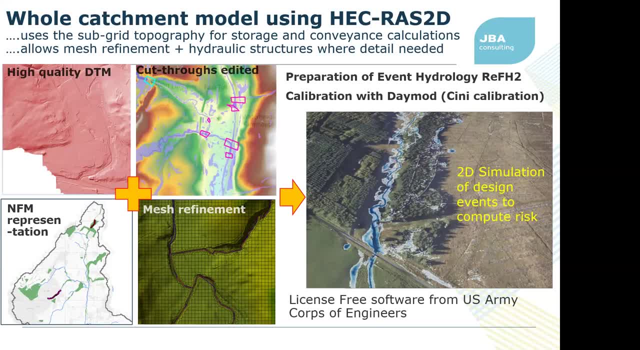 culvert and we do that in some of our work Here. they are represented with cut-throughs And of course that has its own implications for uncertainties in terms of the local airflux near to a lot of detail. and then on the bottom left we've got how do we represent the nfm? and i mentioned 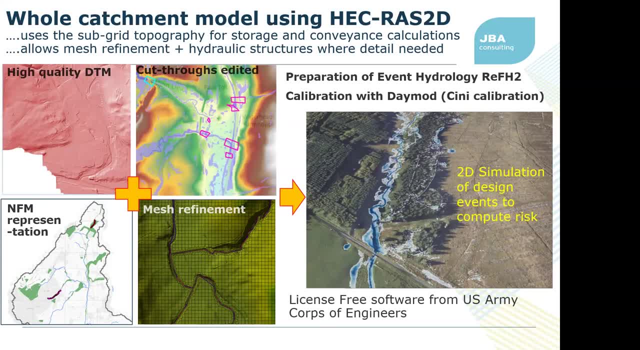 earlier that there's three nerd funded projects, including the qnfm project at lancaster, that nick chapel's leading, martin evans's project in manchester and the landways project down in reading led by joan clark, and actually um, at least two of those are trying to quantify the shifts in. 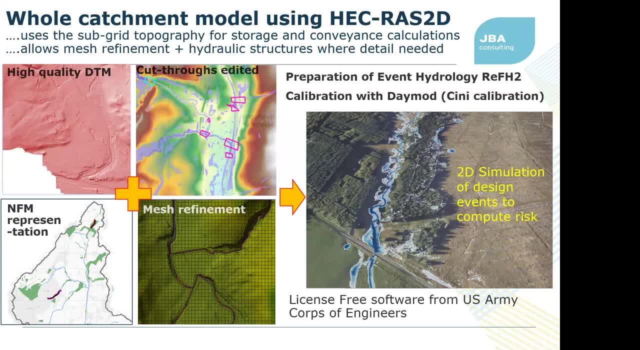 parameters in in models such as this that are justifiable on the basis of the evidence, and we'll have seen from the dadson paper in 2017 about how the evidence, in terms of monitored evidence, suggests that at 10 kilometers squared, we might understand the effectiveness of nfm in terms of leaky barriers and woodland and storage and so on. 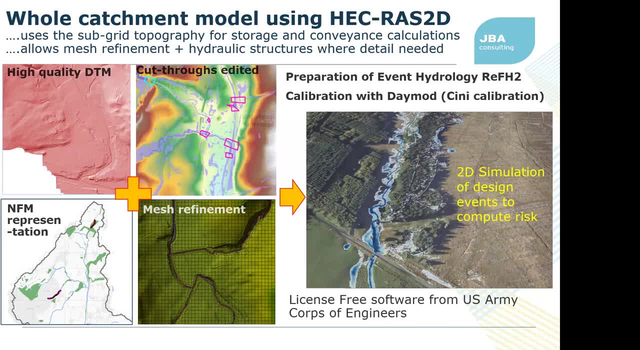 um, but as you get greater than that, the noise in the system, the environmental variability means that it's very difficult in a larger catchment to understand that change resulting from, and attribute it to, the nfm and how you then translate that into the parameter shifts that you use in your model, such as changing the friction using the manning's roughness. 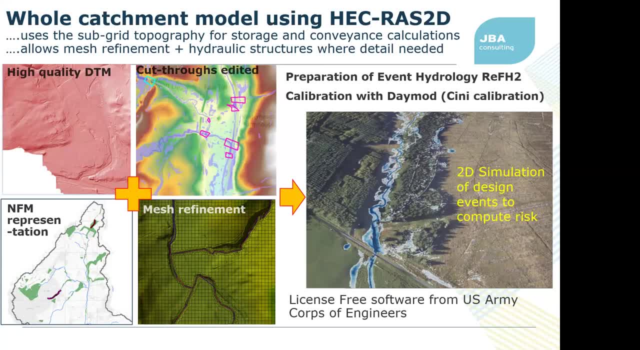 and then, if we move over to the right, the lower right mesh refinement diagram- um, you can see what. what we have to do in a model like this is also, um, what we gain by the efficiency of having this nice sub sub grid topographic representation. we also have to add a bit of 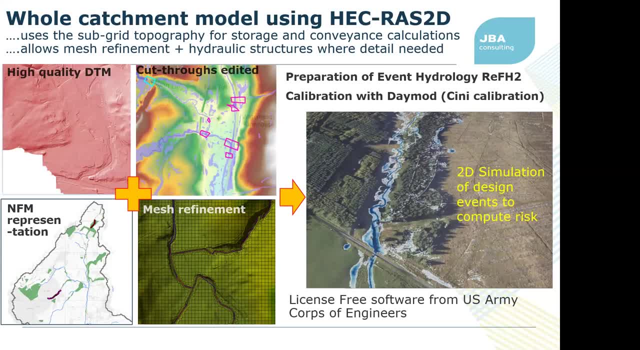 complexity in terms of representing embankments and major flow paths. so you might want to refine the mesh around the channels or around embankments, ensure that we're not getting flow passing through major embankments or convexities. i shouldn't, and that itself can be quite a time-consuming job. but if we do that and then 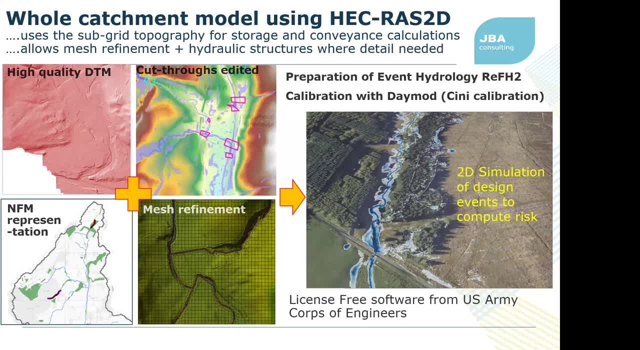 we also prepare, if we move over to the right prepare, the event hydrology. and what we're doing here is we're using the day mod software or the cne calibration utility for fh2 and once we, if we manage to prepare that that successfully, um and understand the antecedent wetness in the 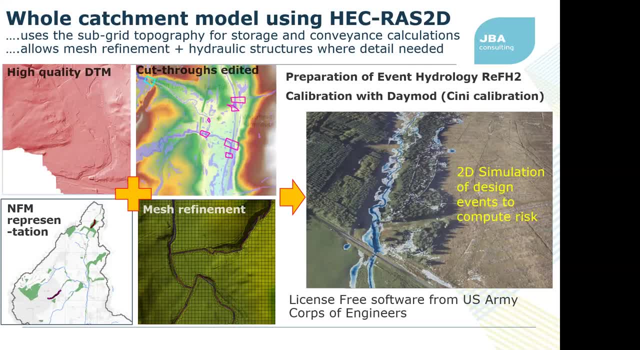 water. we've done that work and we've also planned out what we would define as the moving efficiency for rat doom. but for advanced learning we've covered so many parts of that, which is the memory. we need to sort of justify that. it might look very photorealistic, but how well does it perform in? 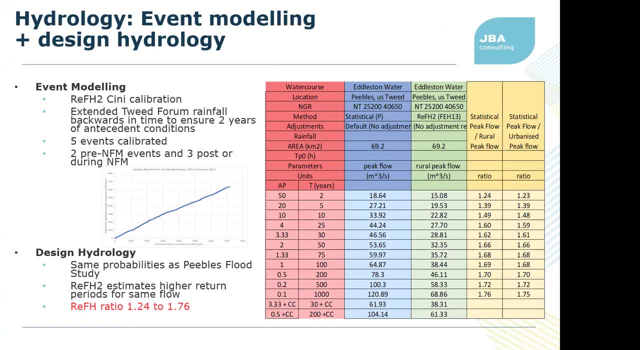 reality. in terms of the hydrology which i'll move on to next, we did some event hydrology, event modeling and design hydrology, and i'm sure there's some very fine hydrologists listening today and they'll probably notice straight away that we have quite a discrepancy between the 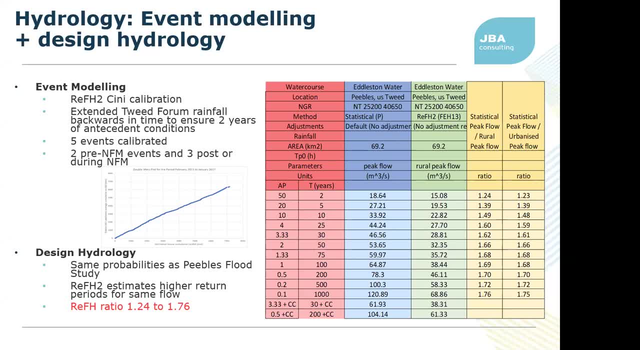 fh to estimates and the statistical method estimates of the design hydrology. we so just going stepping back a bit looking at the event modeling. we use the fh to calibration utility. we had to extend the rainfall from the tweed forum back a couple of years. that meant that for the earlier events pre-nfm installation. 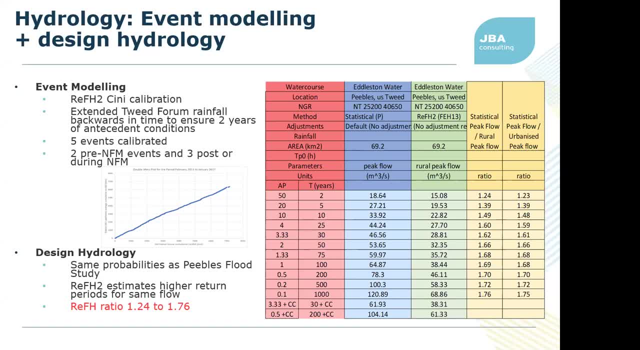 we did have to tie into some more, less reliable data if you like, but we were able to do that reasonably satisfactory and provide two years of antecedent conditions and evaporation data. so on the on the right hand side you'll see those sort of ratios between the two. 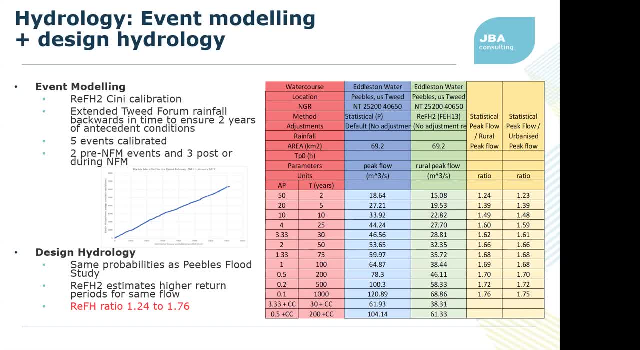 methods and you can see there's quite a lot of uncertainty there, but there isn't that. it's not really been a long-term gauge catchment. so prior to 2012 there might be a level sensor for warning, but there's no. there hasn't been a sort of long-term record of like and the best gauge. 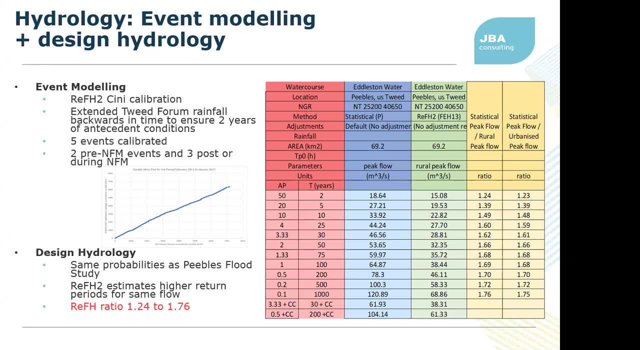 from the swede forum that we have is the kidston mill gauge which has is the furthest downstream with a rating in people's. so there we had sort of typical problems with hydrology. sort of underlines the uncertainty in that for a ungauged catchment that's no longer engaged. 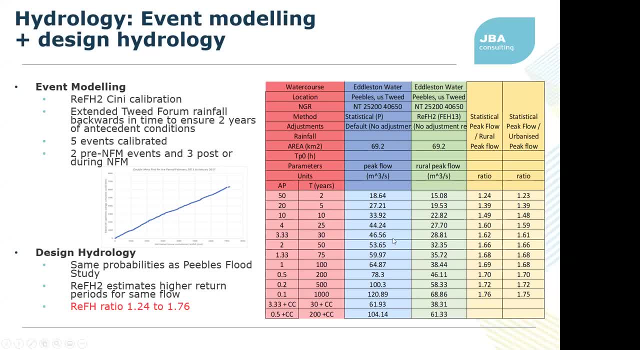 and if i just step on, we. so essentially we took forward the ref h hydrology and we have all the flows. so if we ever need to revert that back to understanding the annual exceedance probabilities, we can do. we can see the process that we went through for some of the events, whether it is 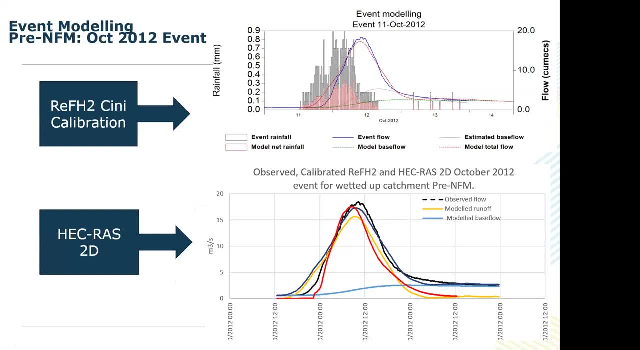 for the actual, real events. so, pre-nfm, we had three events that we looked at and this is the best of them, unashamedly so. we had a june 2012 event and a july one. the gene one did have a trash line survey for a small part of the catchment, which we- although we didn't get such a 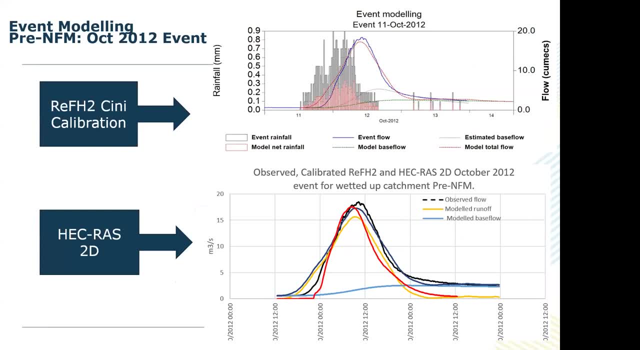 good fit to we. we were overestimating the peak flow. we still compared the outline and i'll show you that in a minute. there, from the first plot, the ref h2c, any coloration, we allowed the base flow parameters to see, parameters to vary and you can see the original and the fitted base flow are there in. 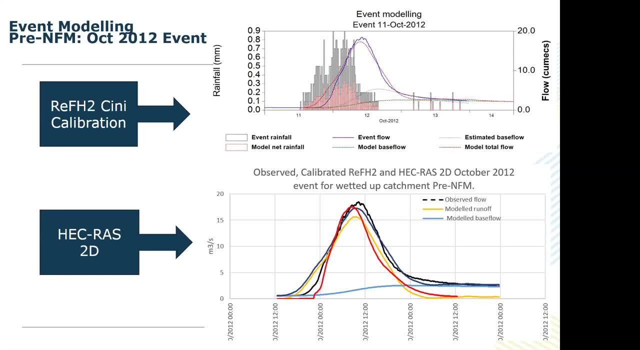 brown. you can also see the rainfall and the height graph and then the net rainfall in red and you can see the data for the event at custom mail in blue and you can see the fit from the hydrological model in red. so that's what we then trusted and we took forward that. 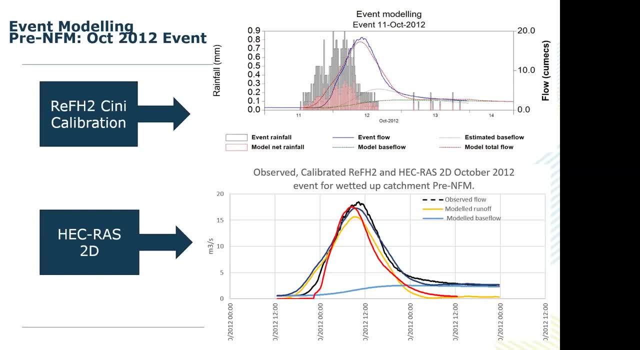 net rainfall and inputted it into as a across the whole of the mesh for the heckos 2d model as a precipitation boundary. of course it would be nice to distribute that and at the moment, although the software is free and has all these other benefits, it doesn't have the distributed 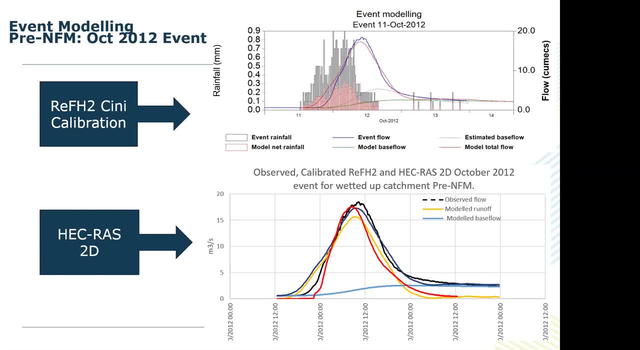 hydrology yet, but that will be coming in version 5.1, which was due to be released this month. um, and you can see what happens when we add that. so if we look at the hydrograph, we can see. um, here i've i've missed out the red uh hydrograph there on the lower plot. 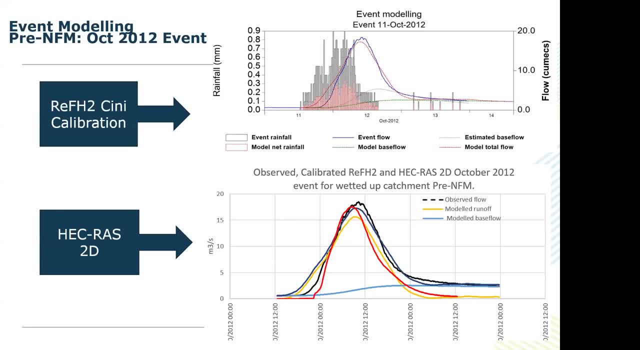 which is the uh hecarus 2d input, uh, simulation, sorry, and um, essentially that's before. we've done a little bit of calibration, uh, sort of calibration, uh, in detail with the roughness, but what we can see is also the model base flow and it depending on where you brought that in in the domain. 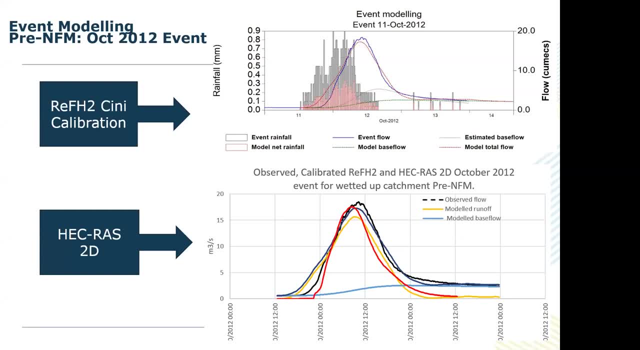 to understand the full runoff, the full hydrograph, and we could see that we could shift the timing of that peak, which isn't quite right. so we're doing very well on the um, on the absolute magnitude, brilliant. so then, what we did was we actually brought that base flow in, uh, along the main stem. 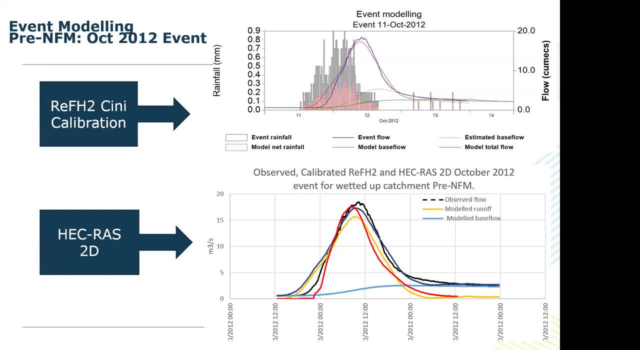 of the river, um, uh, you as an internal inflow boundary, uh, which you can do in headquarters, so it has that flexibility to be adding these, these different boundaries, and then we took that approach forward. so it's probably about as far as you can push this direct runoff and losses approach. 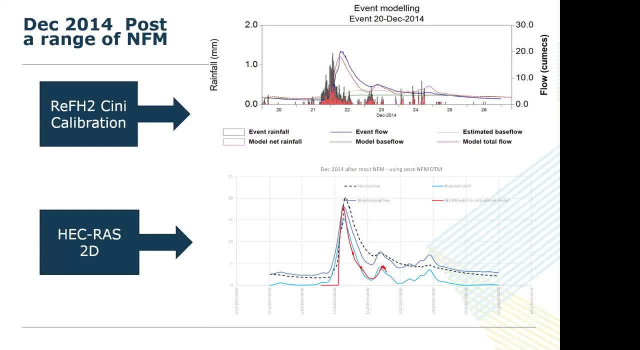 you can see here for another. actually this is a post, a range event, fm, uh events and it's not quite as well modeled. um. we can get the uh. we're under under predicting the flow peak slightly, um and uh, depending on whether we add in a base flow or not. 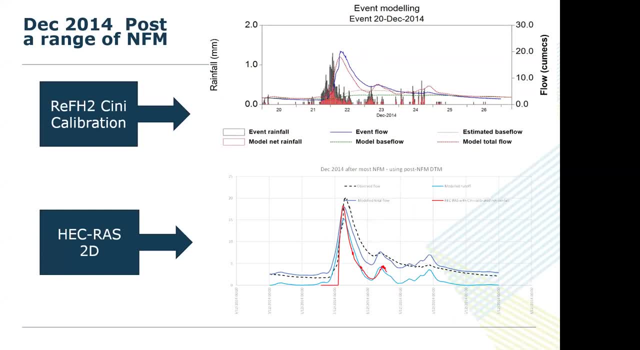 you can see that, um, the start of the simulation is a bit later and in the red plot below on hecarus 2d plot, um, we can see that we sort of get some aspects of the recession and the secondary event quite well there. uh, and it, and this is before calibration and before we've added a base flow in as well. 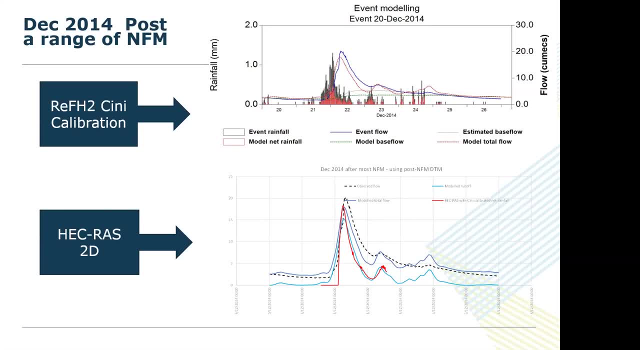 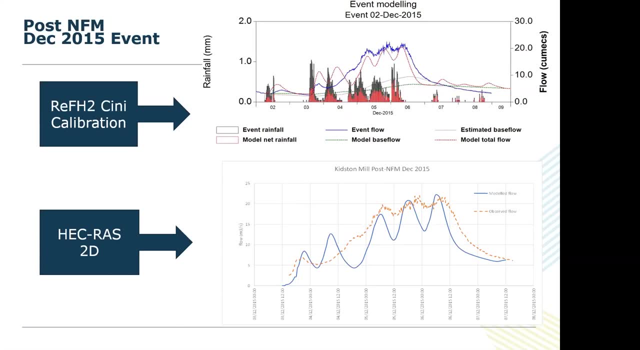 so you can see that essentially we're getting a reasonable you know gave you a bit of confidence that the approach is going to work. now for the post event. as i mentioned at the start of the introduction, um, we didn't have a single peaked event, um, so it kind of exposes a few, uh limitations. 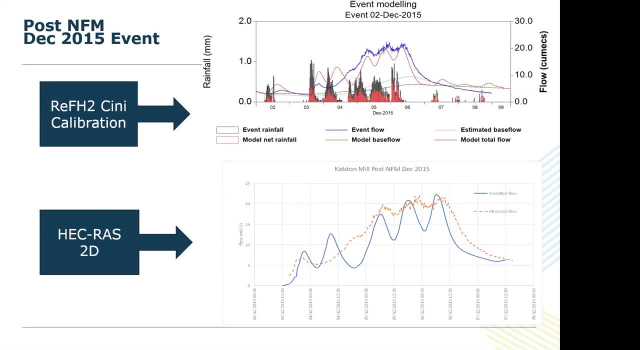 of the approach, i suppose um, but it also um gave us a bit more of a challenge. so you can see on the top again we've got the ref h, two fitted net rainfall and base flows and we can see that the overall fit is the red dashed line. 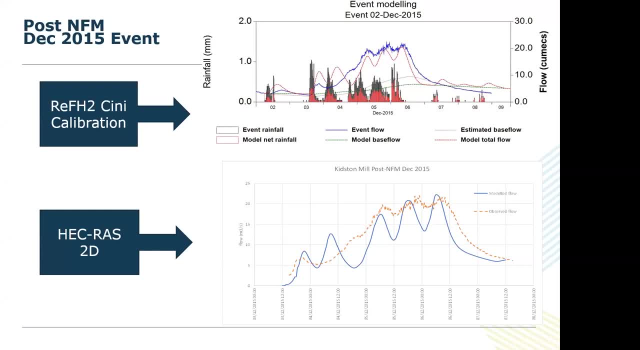 and model total flow and you can see the data. with some noise there, which is to be expected, i mean, on a good day, a well calibrated or well rated flow estimate might come, might be within 10 um if you're lucky. so essentially we're getting up there and you can see the hecarus 2d calibration. 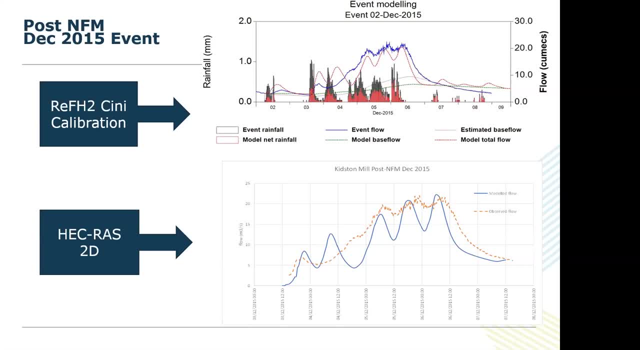 i've cut out more of the intermediate stages on that plot below and you can see this is the kind of level of um fit we can get to that multiple piqued event. other parts of the catchment. there is more sinus to those three peaks um you we're obviously not getting some of the memory term there. 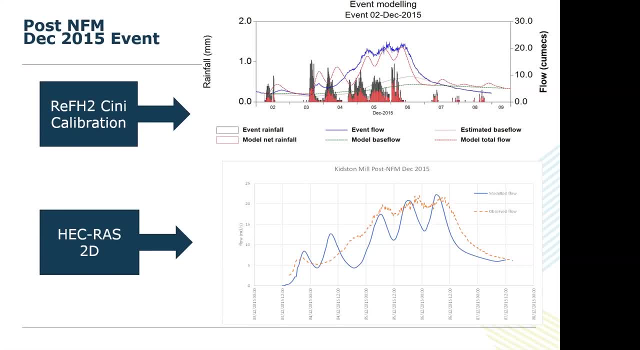 which will be from more of the groundwater processes. that's in the observations in the orange dashed line. But in terms of understanding the peak flows, you can see that we can start to try and calibrate. We're still getting some timing out, but perhaps this is as far as we 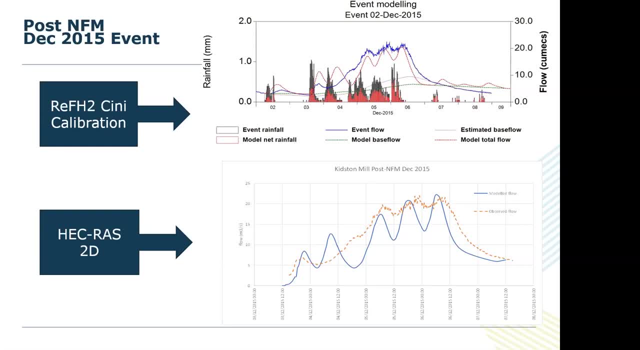 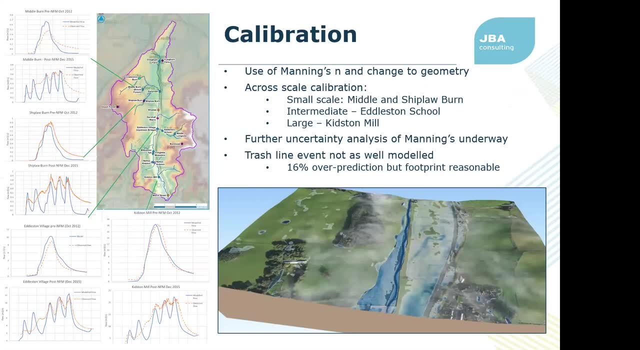 can go without having a fully integrated model. So how did it look across the entire catchment? We did then do some calibration of Manning's N, so rather than trying to represent any of the individual NFM features at this point, we're representing them anything with changes to the. 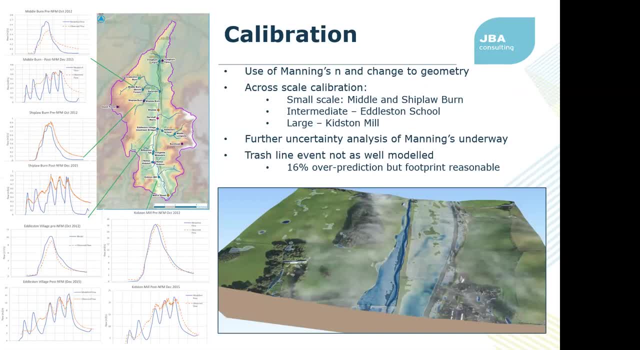 time. We're representing them anything with changes to the time. So rather than trying to represent any of the individual NFM features at this point, we're representing them anything with topography, with a DTM or with changes to the Manning N. So, starting on the top left, you can see. 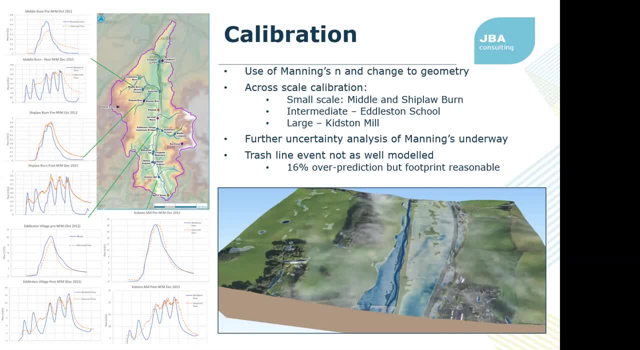 two inset hydrographs of a middle burn and you can see that the pre-event- we're overestimating the orange dashed observations there. This is the best we could do whilst maintaining a reasonable fit around the catchment. As you can see, at some of the other stations we're under predicting slightly. 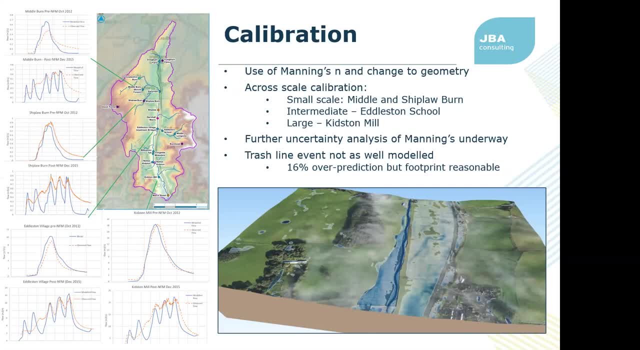 And it could be down to rainfall input differences which we can adjust when we have a variable version. You can see that for the two small scale calibration sites that we looked at- middle burn and ship flow burn- we get a reasonable fit And for both of them, for the post-NFM December event. 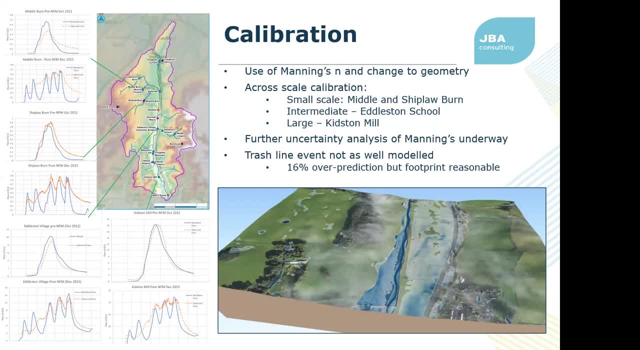 we're getting the peaks about right And, as I say, I think that's about as much as you can do with this type of approach. And if we look sort of partly further down the catchment, so the intermediate scale. so here the 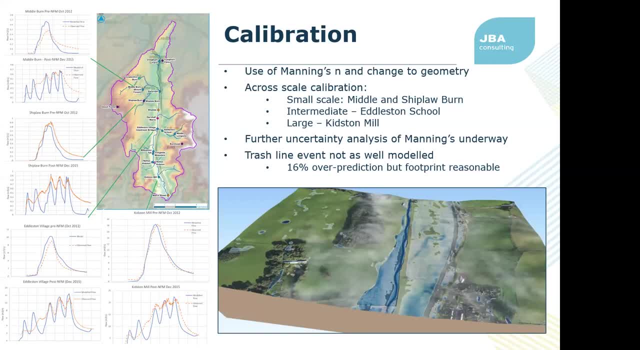 catchment area might be about 30 kilometres squared instead of 70 for the whole catchment At Edelston Village. we can see that we're getting, if you look inside the model, we're getting a reasonable fit as well. So the bottom to left inset hydrographs show: 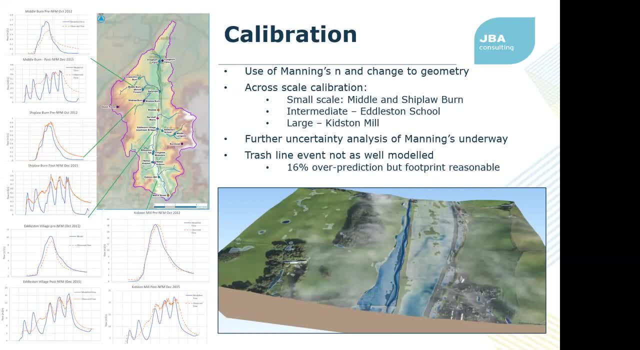 you the slight over-prediction for the pre-NFM event, which was 2012.. And then again a slight over-prediction, but not too bad, for the triple peak. In fact, here you can see that the data is also showing a greater degree of variability than higher up the catchment. 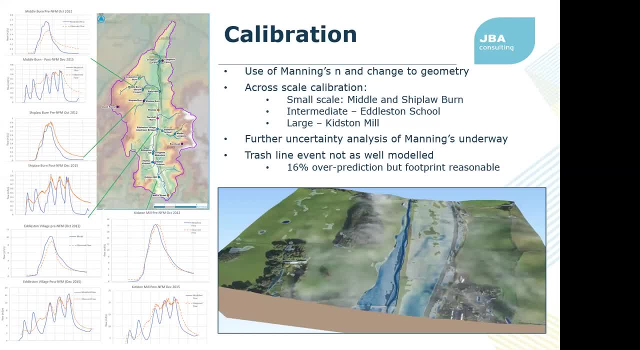 So I think here maybe the conveyance is dominating over those groundwater inputs that give a more damped response higher up And then at the very bottom of the catchment. so this is, if you like, the sort of whole catchment calibration point down against the 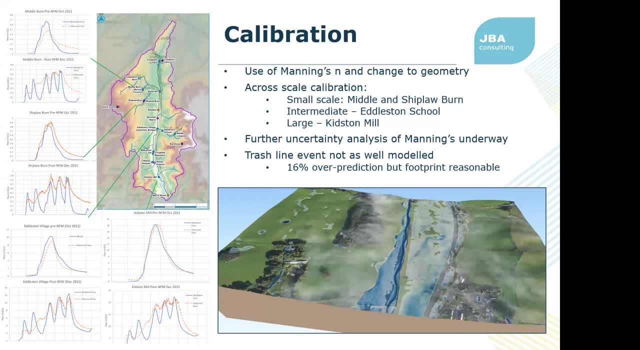 mountain because there's no rating. at March Street in the orange we can see the kind of level of agreement in terms of the peaks. So had we had a, we probably have now had a decent post-NFM event. we might end up with some calibrations that are more. 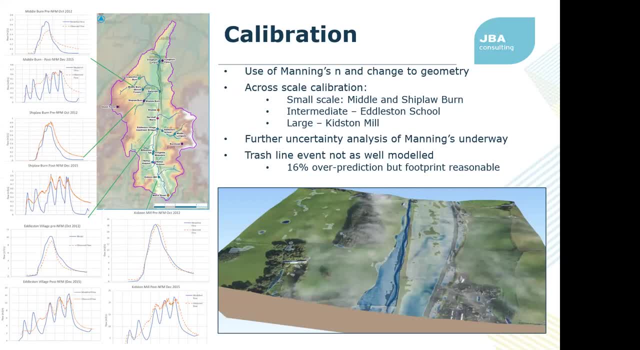 like the pre-NFM you can see there And this kind of oscillatory behavior which doesn't make it easy to model and look at before and after And then. so, as I mentioned earlier also, there's a sort of further uncertainty analysis into sort. 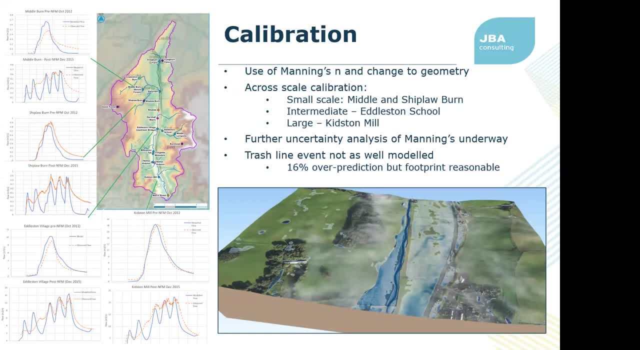 of varying the distributed Manning's roughness representing the NFM. Now, of course, that will change through time, But I think it's really important to look at the NFM and I think it's really important to look at the NFM, and I think it's really important to look at the NFM. and 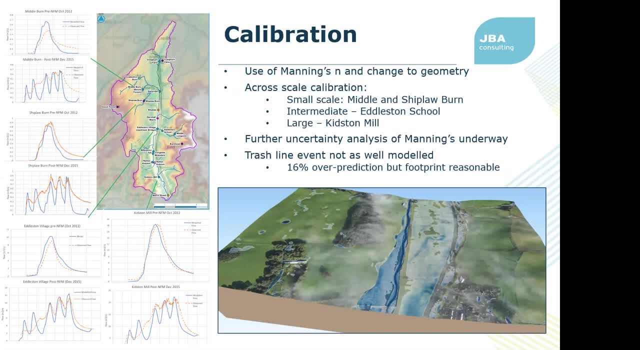 I think it's really important to look at the NFM as well and it'll have its seasonality, So as the increased roughness that's already been generated has been calibrated. but as we go forwards over the next sort of 10,, 15,, 20 years, I understand you get kind of a canopy closure. 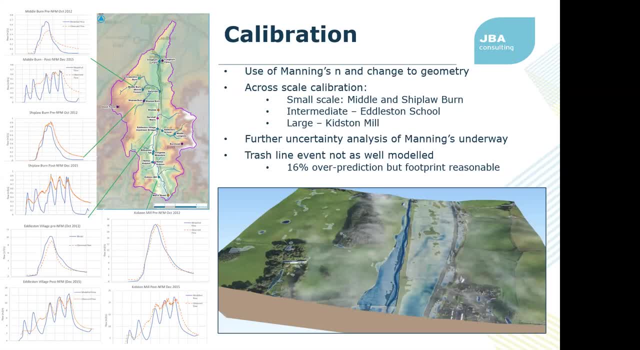 around about 15 years, and then we could, longer term in the future, have those woodlands generating woody debris and creating little debris, dams and so on, And that will increase the sort of slow. it will slow the flow. So through time we'd expect these values to change. 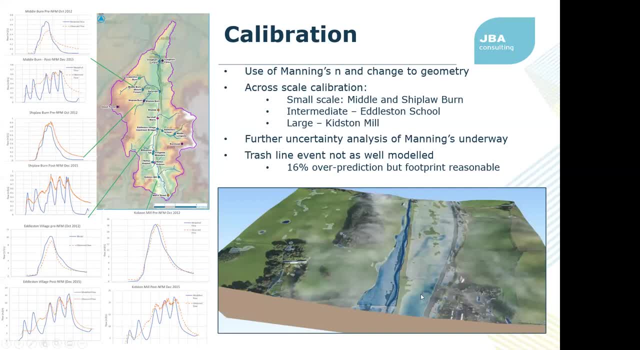 So there you can see the bottom right. we've got the only sort of spatial footprint from a trash line survey, which is the kind of darker blue area on the left hand as you look at it. So for that event, we captured it. 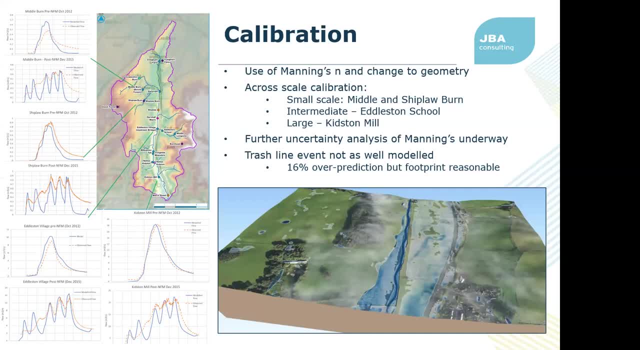 but we were over-predicting and in fact the extent is slightly over-predicted in the upstream end. You can see that better in a less 3D plot, but I quite like showing it like that. So again, a bit of confidence. So is this the best we can do with this type of approach? 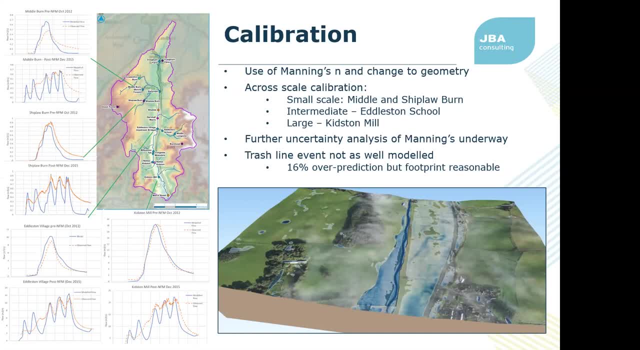 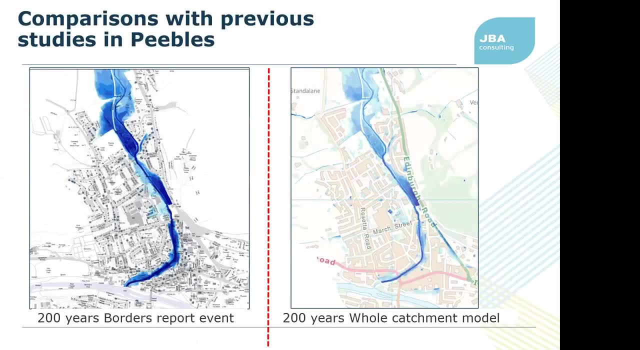 Perhaps we could work on it a bit more, work on the mesh in a bit more detail and use more distributed hydrology as well. We made other comparisons with previous studies. So in Peebles itself there's been a Peebles flood study report. I didn't have all the details of that. 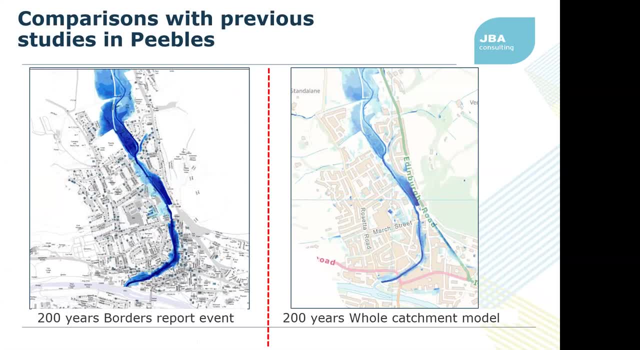 but we have here a sort of outline, a depth grid of the 200 years report event And we're getting something very similar with this whole catchment model which takes into account all of those, as I mentioned, nearly 300 million pixels. But 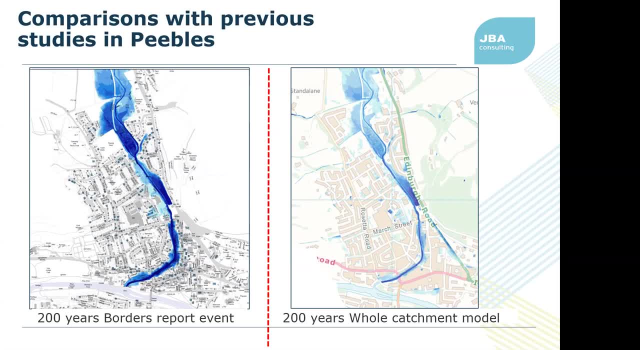 we did get some differences. The color scale is not quite the same here but we can see that in Peebles itself we've got quite a bit of distributed surface water runoff We've got. if you look further down the Edema Road we've got more water accumulating along that than in the other fluvial model because 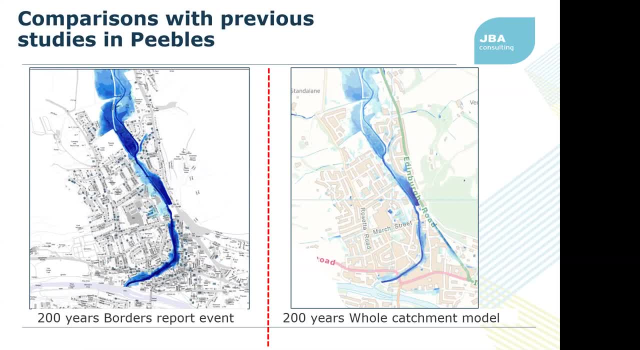 that was built using a more traditional fluvial approach, Whereas of course here we've got direct rainfall to the DTM. So we can't quite make an exact comparison between the damages and the estimated annual average damages between the two. but we can look relatively And we'll do that slightly further on. 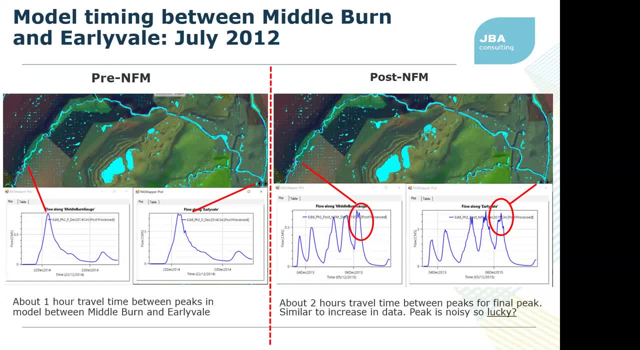 So we're starting to sort of get into the bones, at meeting bones, of trying to understand. if you've got a model like this, can you start looking at things like synchronization of peaks around the catchment? Can you start looking at things like synchronization of peaks around the? 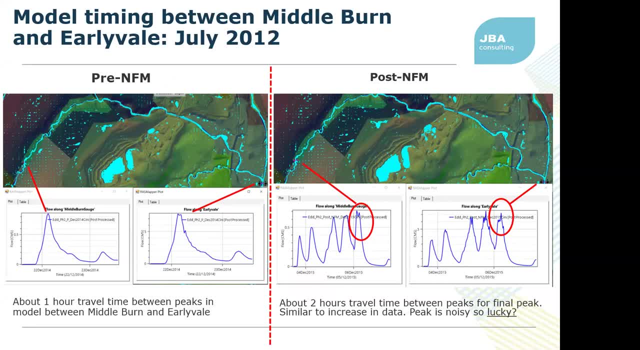 catchment. Can you start looking at things like synchronization of peaks around the catchment? Can you start thinking of the model as giving you a representation of the whole system, Because that's what ideally. this would be useful for sort of understanding how all 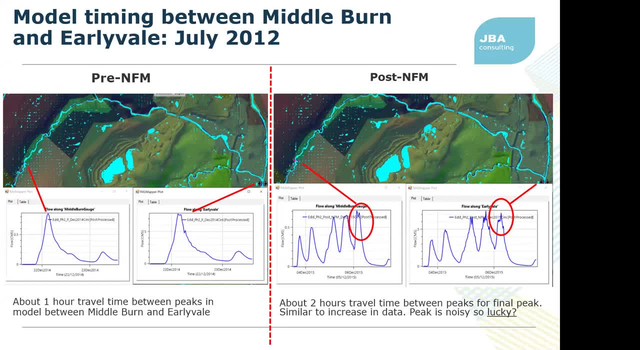 that water's been pushed around simultaneously if it's driven by rainfall, rather than by some imposed FEH or FH hydrograph boundaries. So here, what we found was that for the here we're looking at on the left, we're looking at a pre-nm. 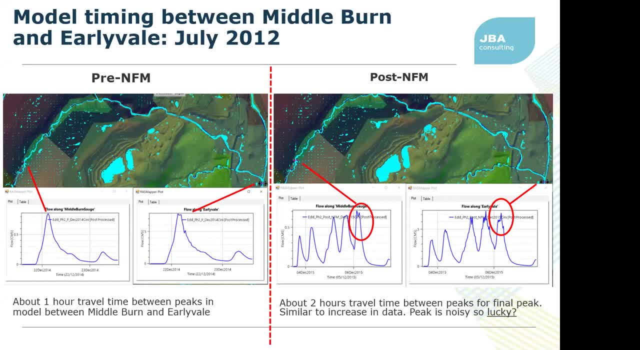 or it's actually a sort of post. it's the 2014 event And the difference between the time of travel. sorry, the time of occurrence of those peaks was about an hour And on the right about two hours, and it agreed largely with the data analysis And that was for the December 2015. 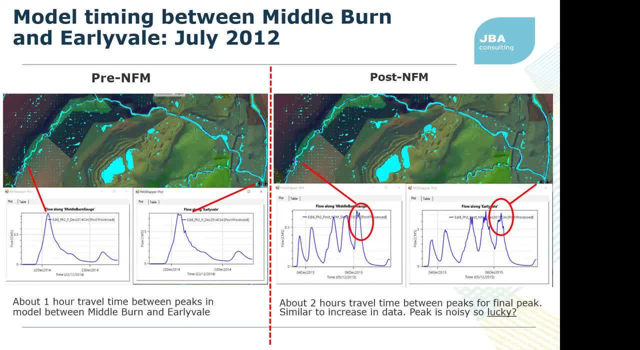 analysis. So yes, but you can see that are we being a little bit fortuitous with the data there? There's a kind of noisy re-peak at the end of the 2015 final peak And similarly on the left-hand panel of that one. 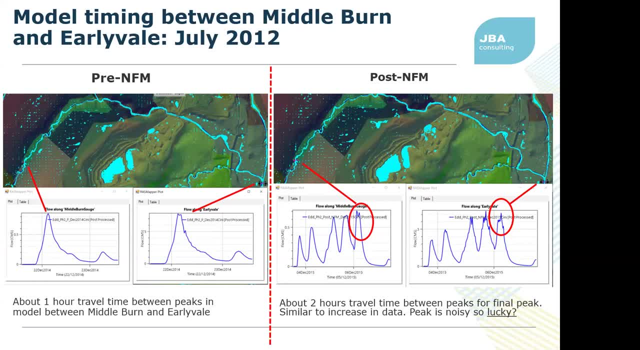 you can see that there's like a little double peak. So in some respects, yeah, we're kind of understanding what's happened with the timing between sites, But perhaps in this instance, with these events, it's fortuitous and it'd be nice to look at more. 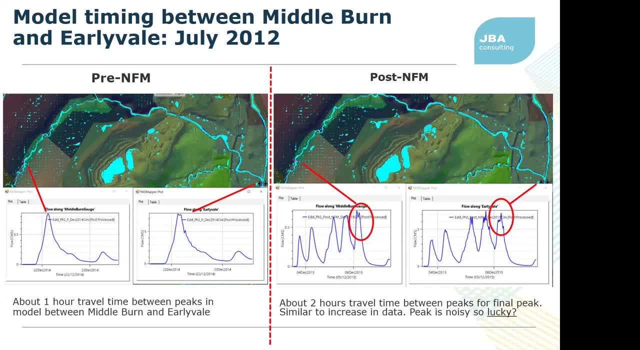 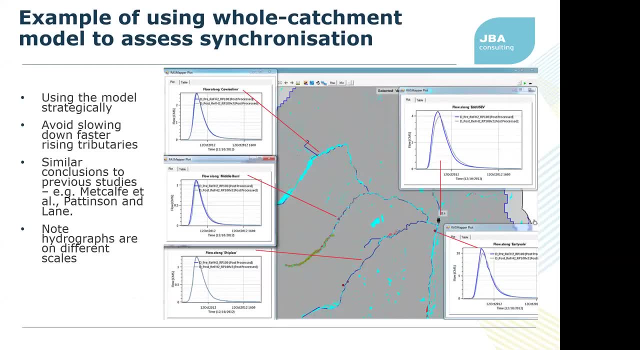 And Dr Andrew Black is analyzing that, the timing over many more peaks to understand what it means statistically. So okay, well, let's try and understand if we could use this model to understand synchronization, as others have done And I've zoomed into this, is using RAS Mapper. 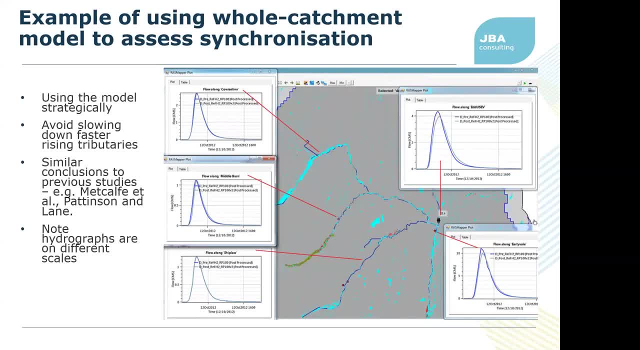 which is kind of shows some rather chunky depth grids before we've kind of mapped back onto the one and a half meter DTM And the three tributaries. you can see there we've got Caris, Linn, Middleburn and Shiplaw on the left And on the right we've got we've got Eden Vale. 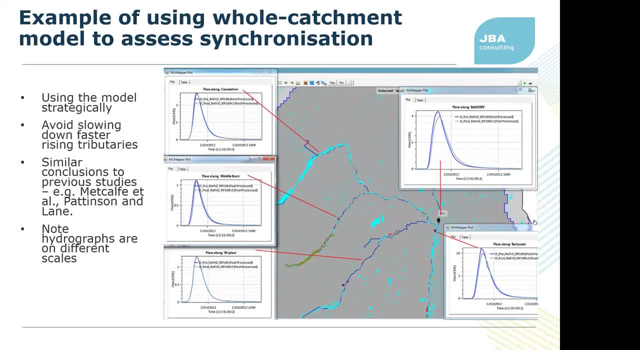 and we've got upstream and downstream of that confluence. And so one of the things that stands out here for this 100 year design event- and this is one of the final events, but it's kind of- is that we've got some sort of small changes in Kerry's, Lynn and Middleburn. Not a lot going on. 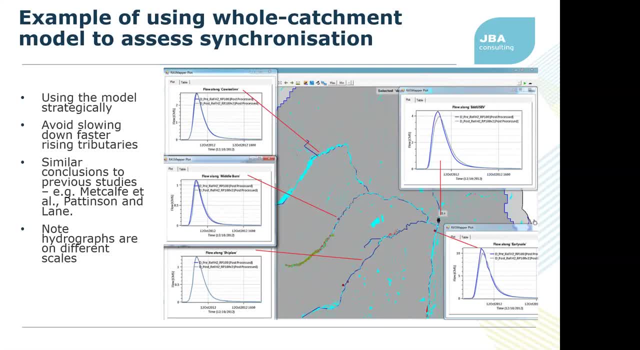 ship though, but then perhaps we wouldn't expect that yet, because that's purely native planting. But as those join the main stem near Early Vale, we have a change in the peak which is more significant than it looks, because the hydrographs upstream and downstream of that confluence 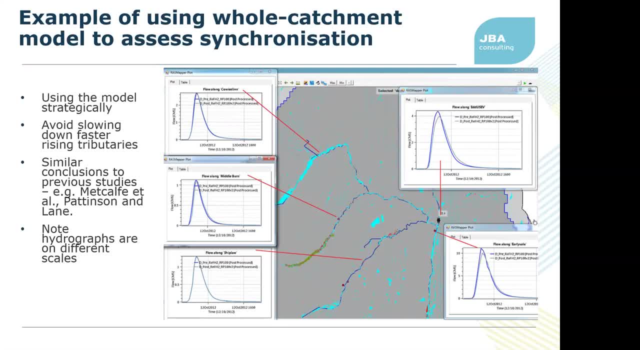 are on different scales, But the timing hasn't really changed much from the upstream one, and so the question is: would it be better just to slow down the slower rising peaks than slowing down the mull? And then that question came up in a number of studies. There was the Peter 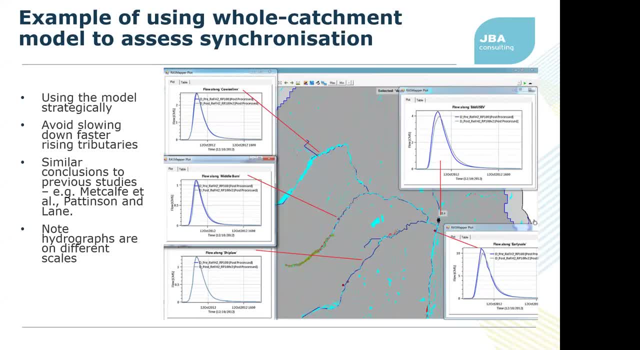 Metcalfe study in the Brompton catchment and then I know that in Paterson and Stuart Lane did something similar in modelling the Eden. So yeah, I think if we're doing quite a big bit of change within the catchment then the understanding of the timing effects is important. 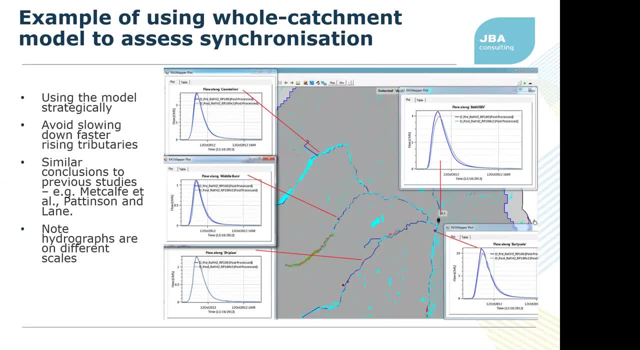 And it might be as well that you know we use this model. now it's set up to understand that in more detail, so we could have some what-if scenarios where we do an awful lot on the left-hand tree, which is there, and nothing on the right, or vice versa. 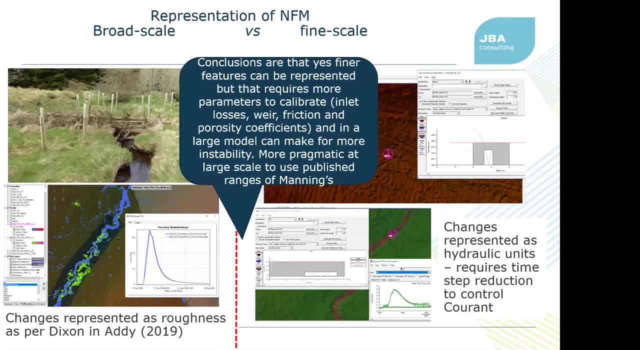 And see where that gets us. Now I'm just going into sort of understanding representation of NFM, which is a very generic term, and here I'm talking about the representation of the engineered log jumps. There's a typical one on the left from Middleburn. There's a photograph from the street forum showing some logs that 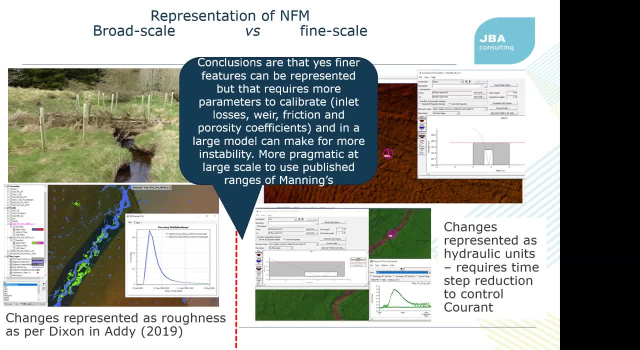 are pretty substantial, but the important thing to note is they extend across the floodplain considerably and there's also floodplain planting And you know, when we're looking at this stream here, we're talking a few fractions of metres cubed per second. we're looking. 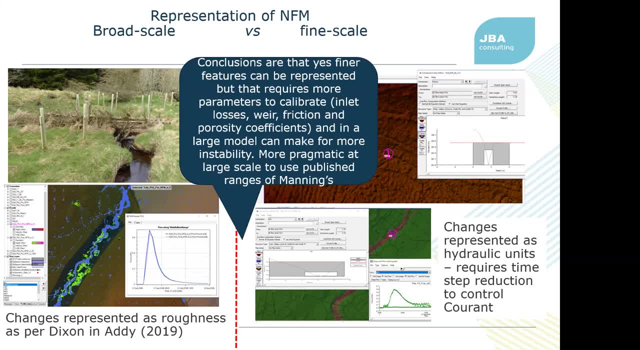 at in these, these peak hydrographs. So that's the kind of order of magnitude And on the left we can see the broad scale representation. if we start representing that whole area as a sort of patch of increased roughness- And there's some nice summaries of that, So you can see the roughness of the log jumps- 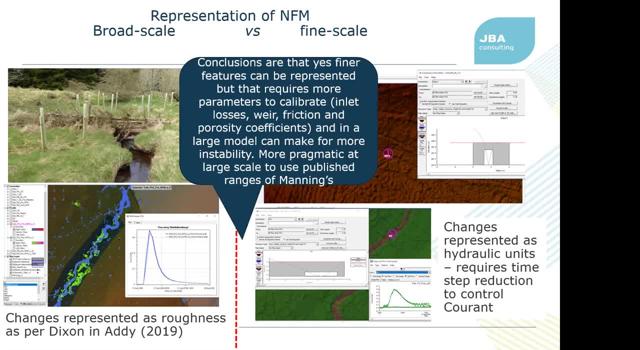 There's some nice summaries of that in the recent ADDIE publication And we have the added benefit of being able to, of not really having to calibrate many more parameters if we start modelling that as a hydraulic feature over on the right, So on the right, you can see there the granularity of the 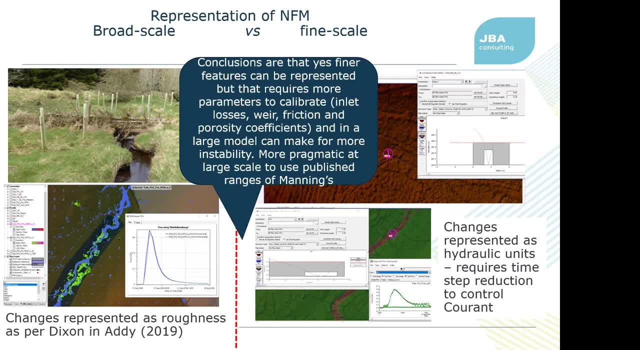 DTM, so it's really quite impressive in places And on the right. what we've tried to do is we've just simply represent it as a embankment with a rectangular slot through it, So the energy losses there will be represented by a kind of Bernoulli effect. We can put in multiple slots to represent. 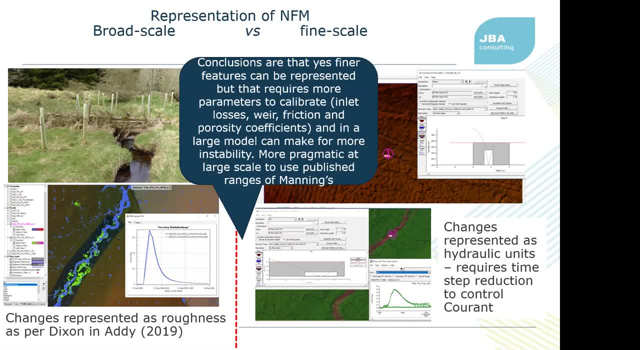 porosity. That in itself is a kind of parameter. The geometry is also something to define. I mean, it's quite an ambiguous kind of shape And we've modelled it with a rectangle And then, of course, with those we've got to have wear coefficients for the flow going over. 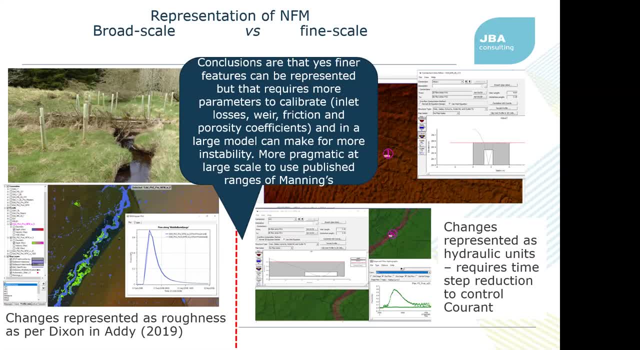 Inlet losses, friction porosity coefficients. So what happens is you can end up with some nice representations of those features, And I think this is really a few important points here is that you can see that we've had to refine the mesh around that feature, And then that in itself 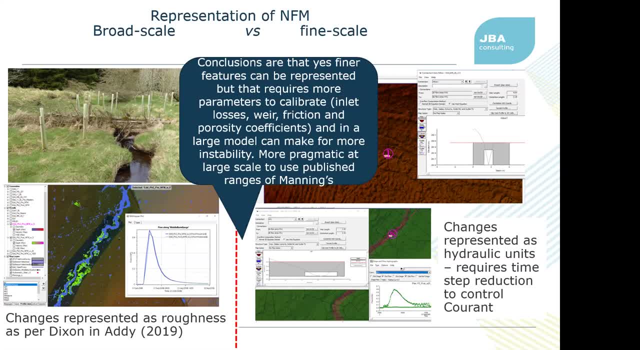 means that you're going to have to start reducing your time step, So the model runtime for the entire 70 kilometers squared then explodes. And also you can get some nice outputs from the geometry view or from rasmapper in terms of the flow through and above the wear feature And obviously you're getting some oscillations. 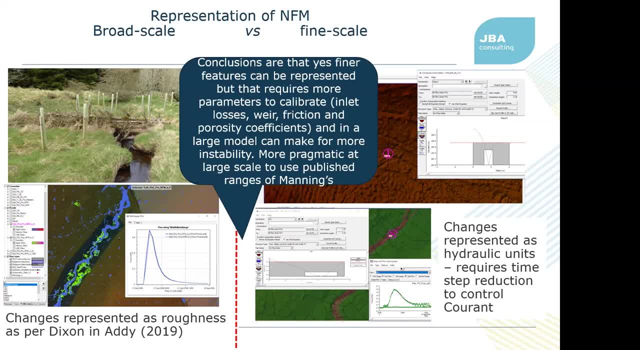 there which could be removed by reducing the time step even more. So you can see that it swings in roundabouts. and it's actually one of the things I think is quite important here And it kind of brings together with sort of thinking coherently with what some of the NERC projects are doing as 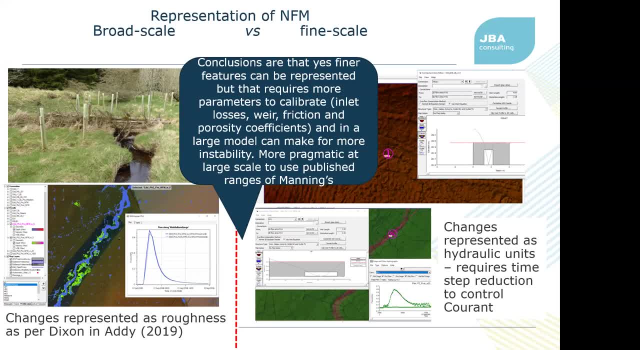 well, Is that perhaps it's more useful to sort of understand what's happening at a very small scale. make a smaller domain model of perhaps a kilometer squared. I'm thinking of Nick Chappell's one kilometer catchments and middle bend here. 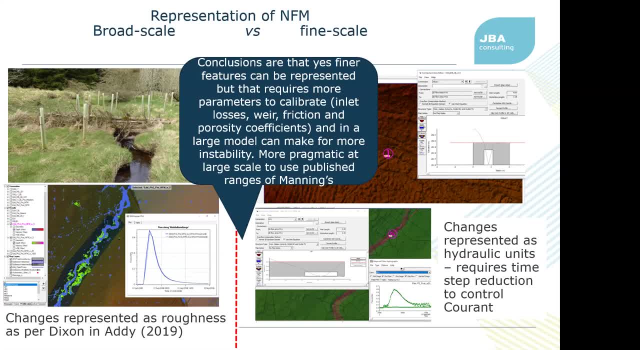 And then, Yeah, And what we can see is that we could model it in detail, we could have sensible runtimes and we could have a hope of calibrating those additional four parameters. But if you want to represent the system at a big scale and understand the whole system, 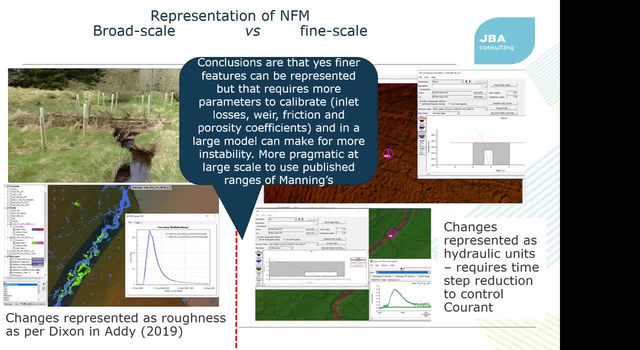 response, then perhaps it's more effective to represent it in a different way and use some of these measured or these calibrated values that are in the literature, as mentioned, And that's what we've done. So that second approach is what the broad scale approach is what we've done in that. 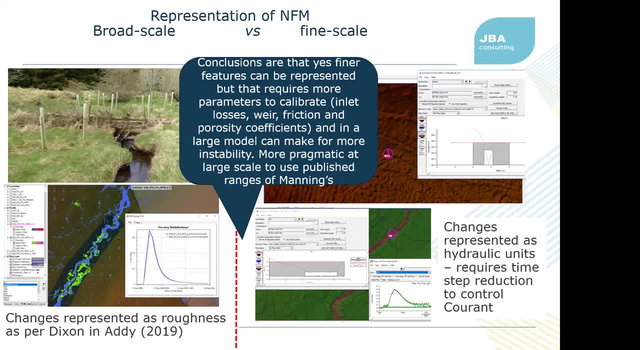 across scale calibration that you saw earlier. Now I'm not saying you should shy away from representing it in more detail. what I'm saying is that it might be better to do a portion of your catchment where you've got a lot of NFM. 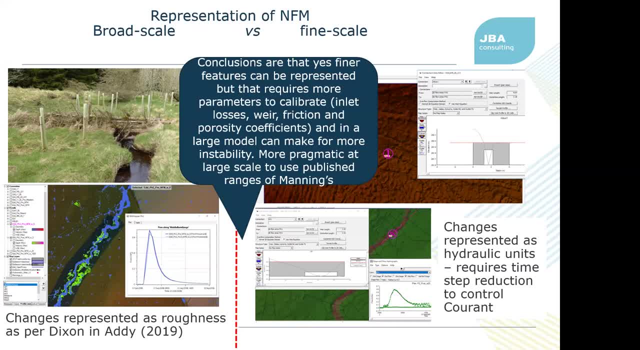 Where there is a big shift in some of those parameters, perhaps where you can hope to detect it and you can also model it in more detail, And that in itself gives people confidence that if they did that everywhere else in the catchment then it would be effective. 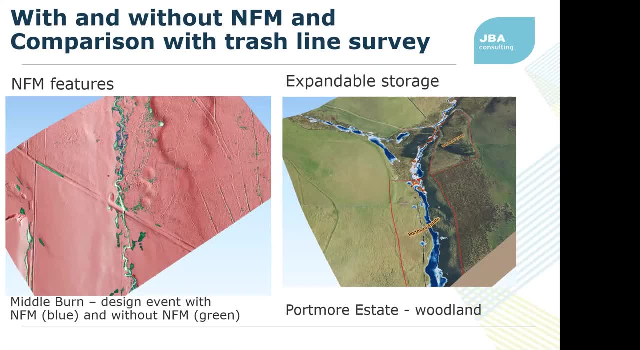 So leaving that discussion for now, if we look at some model outputs with and without NFM- And the reason I've done that here Is largely not to show that you can use QGIS and so on to visualize it, but to try and 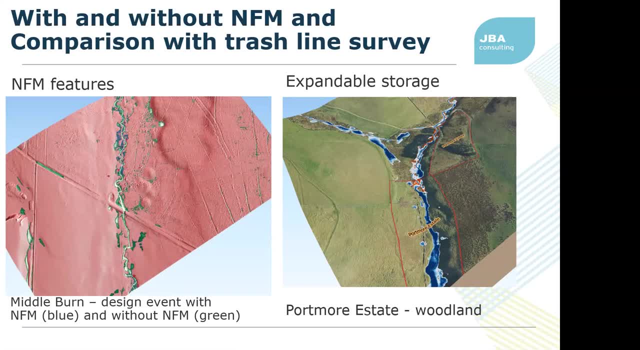 understand what's happening during bigger events and so on, And what's happening as we increase friction or as we build structures like the one we just saw Now. what's happening here, in both these instances, in different sort of areas in Middleburn and Portmore? 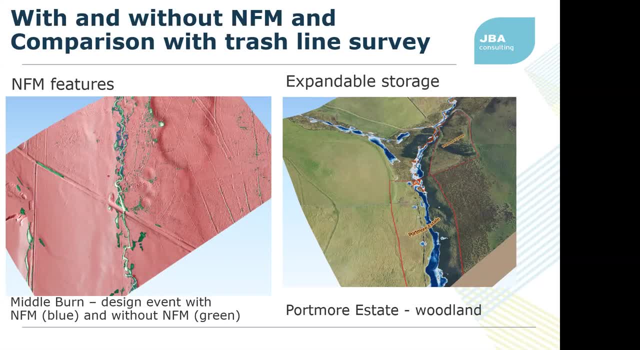 We're pushing more water onto the floodplain, And that's what we're doing, And that's what well-designed NFM would hopefully do, in order to provide more and more storage at bigger and bigger events. And, of course, it's down to you know the timing of that. 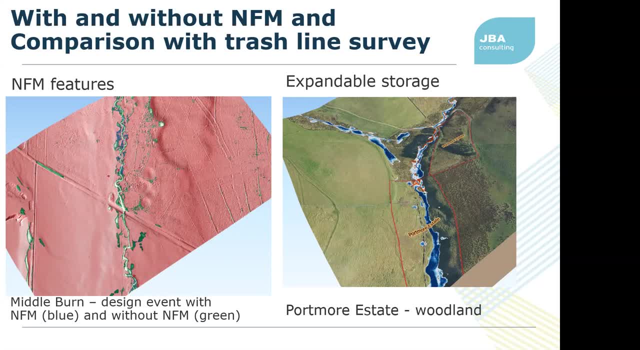 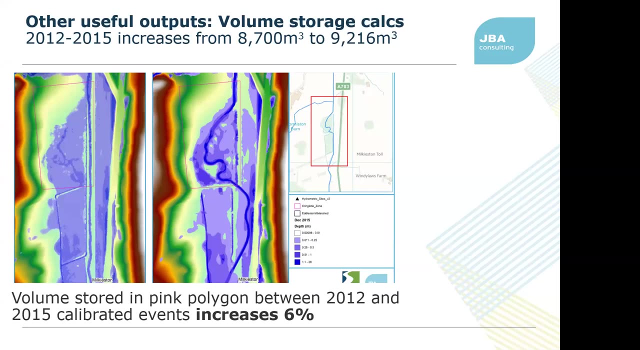 Is it taking that water from the peak and so on, which is where the model comes in useful. So I guess remember what those diagrams look like or those figures look like, and we'll move on to the next slide. So here we've actually sort of zoomed in on an area where there's been re-meandering. 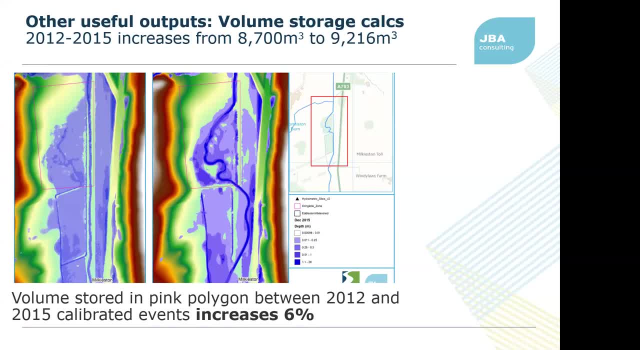 And for that trapezium. there you can see on both of the diagrams in there, both of the figures, you can see the pre and post NFM or pre-meandering, You can see the volume can be computed quite accurately. So. 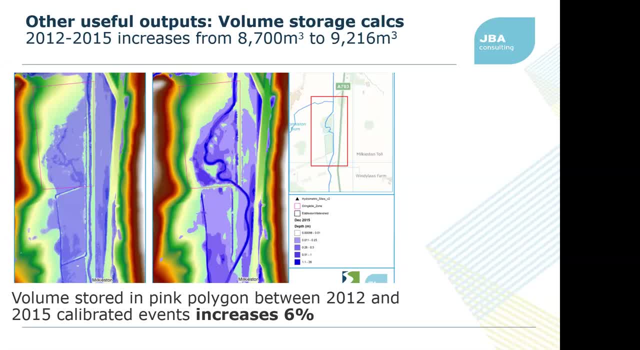 Heck, as I was mapping back to this half meter. it's very useful to be able to integrate that up and understand the change from that work in terms of the absolute volumes that are being. So the volume there has increased by 6% before and after and you know you can compute. 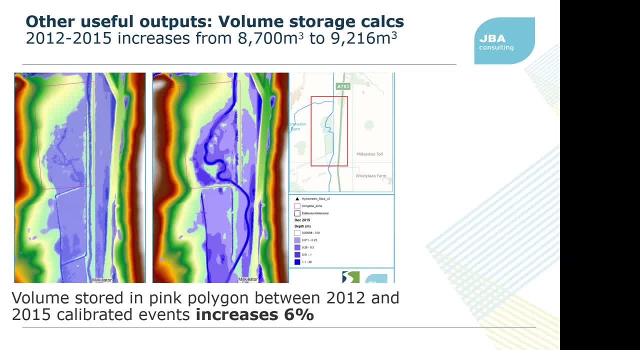 that quite accurately with these kinds of outputs. So so, so, so again here, here, what we're, what we're hoping to do, is we're going to- We're hoping is that more of the water will be stored temporarily and cause attenuation. 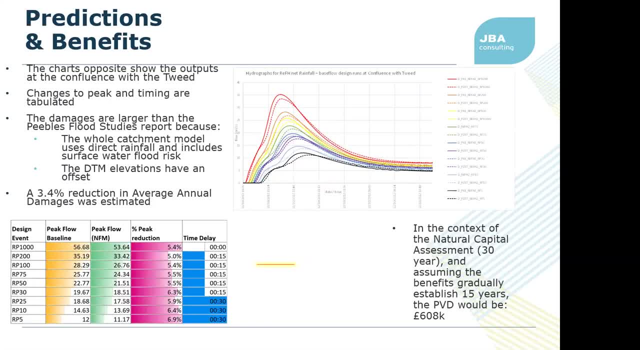 if further downstream. So let's take it that we're happy with that calibration. And let's look at some design events now and look at RefH says So. we've got quite a number of Think it's here, Hi, starting with the top right. 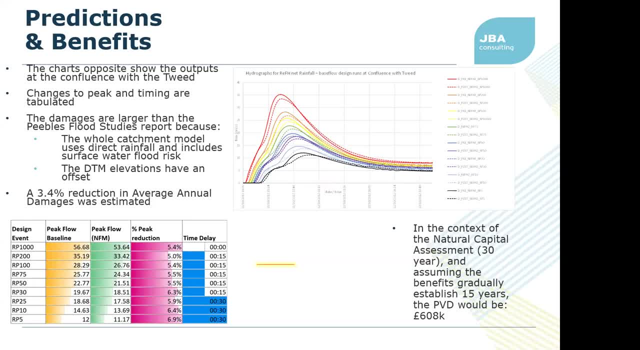 We've got About design events. we've got them with and without NFM. so this time we're purely representing the NFM in terms of increased friction from the calibration and also changes to the DTM which are around places like the Meanders at Quangoletti and so on, And you can see. 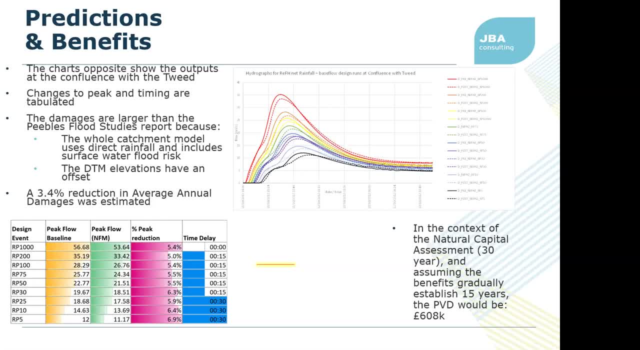 here that something that I've noted in other studies as well is that we can see that those- in this instance the NFM- is being effective across flows which, as the flows get bigger and bigger and bigger, we're still doing something. It might not be a lot, and if you look at, 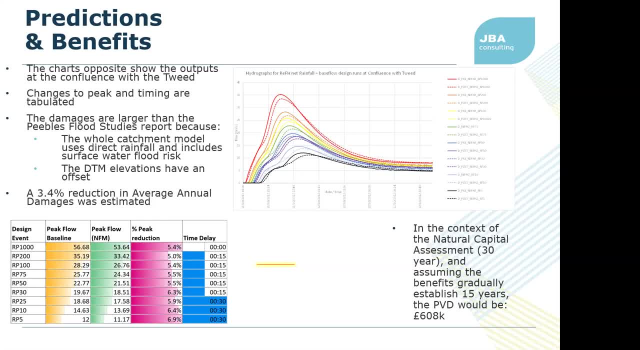 the table on the bottom, the pink bar charts show you kind of that. we're around about 5% peak reduction across flows And now the uncertainty might be, you know, it could be 10% on that, so just bear that in mind. But here what we're seeing is a change of that order And I went looking around the 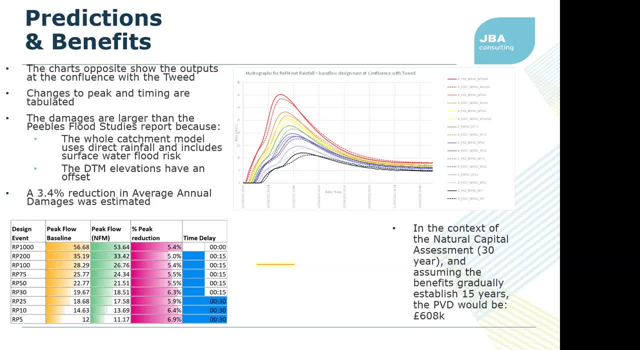 catchment to see why that might still be happening. And indeed, if you look at those locations where you're pushing water onto the plane, some of those areas are more and more expandable. They are You're driving a flow pathway into an area that can accommodate more and more water. 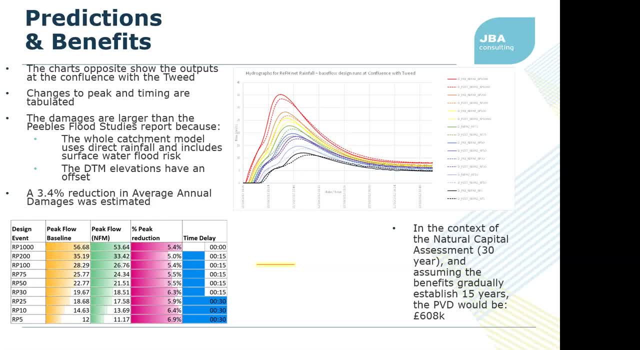 So I think this effect needs a bit more analysis and we've been looking at it in the QNFM project and we've been looking at it also in the Connecting the Column project in Devon, And it's something that gives you hope that, okay, we might not have made a massive change to that peak with. 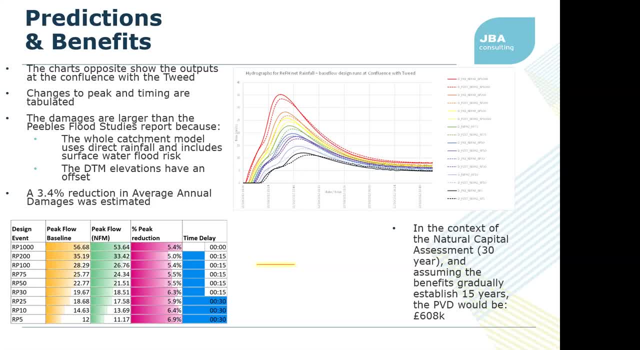 what we've done here. But if the NFM is designed to be more and more expandable, then it's going to be more effective. So I think this effect needs a bit more analysis, and we've been looking at it in the QNFM project. 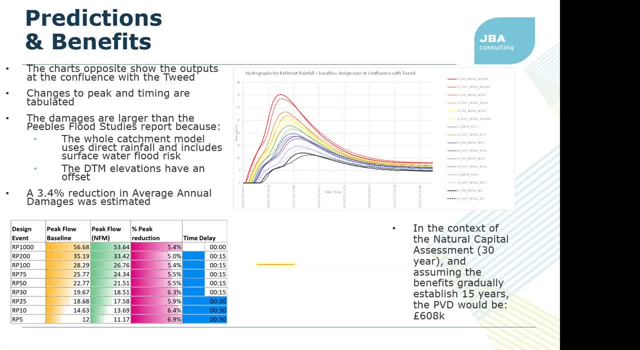 and we've been looking at it in the Connecting the Column project in Devon. So I think this effect needs a bit more analysis and we've been looking at it in the Connecting the Column project in Devon. So I think this effect needs a bit more analysis and we've been looking at it in the Connecting 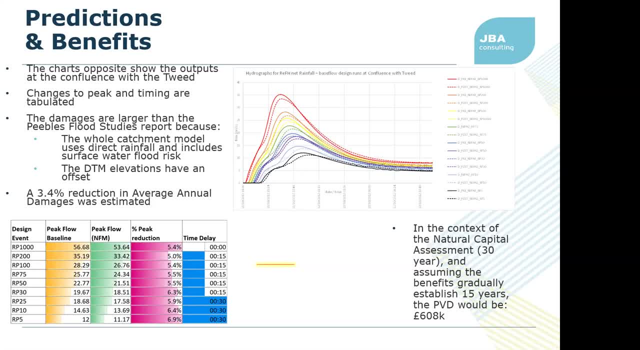 the Column project in Devon And it's going to be more effective. But if the NFM is designed right, it could reduce across different magnitudes And there's a reason, a physical reason, for it. Now, if we go down a paragraph, we're looking at the damages. 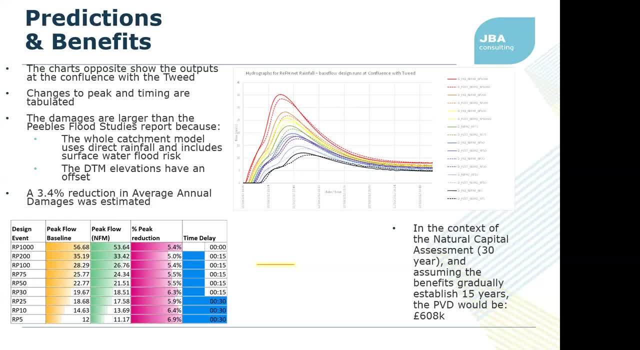 So, in terms of the estimating the damages, the reason why we might look at so many design events is that they each have a probability or an annual exceedance probability, And if we integrate the damages versus probability for each of those, they're going to be very 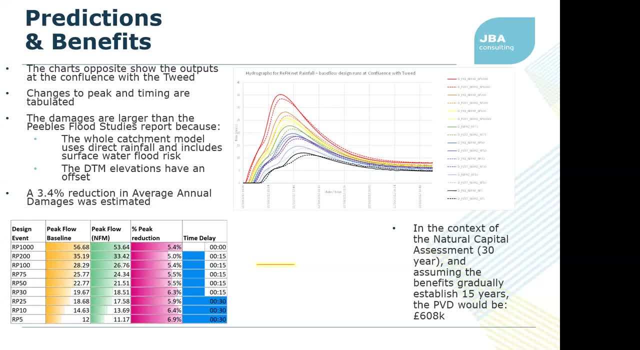 different. we get an estimate of the expected annual damages, or the long-term average annual damages, and the difference between those with and without NFM is about 3.4 percent. so we had a reduction and you think, well, that's not a lot for all that work that I've done. but if you were to 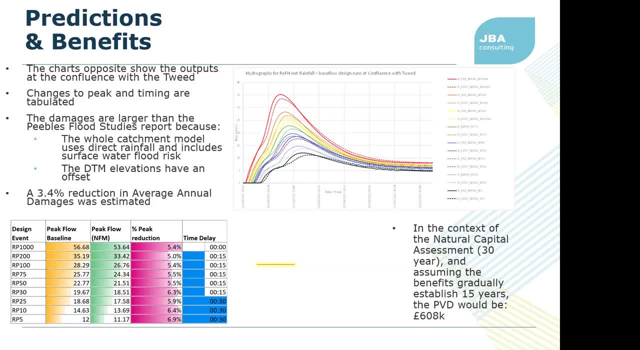 look at that in the context of a whole scheme, lifetime and estimate present value or the net present value. you can see there that we've estimated that over 15-20 years to be about 600,000, so it can be significant and up there alongside some of the other multiple benefits. 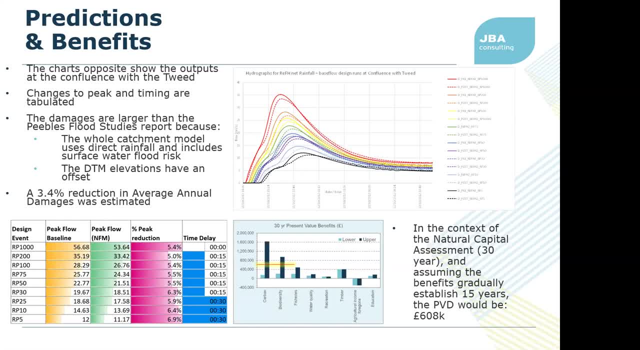 that you get from NFM. so Angus Pettit, who's been the project manager of this, did also did a natural capital assessment for JBA, for the Tweed Forum as well, and you can see there that different estimates of carbon and biodiversity. you can also see the 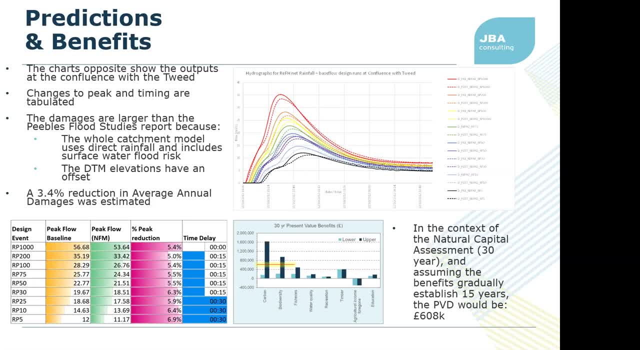 uncertainties there. so he's gone better than me and put a range of values there, and that's something that we'll be, we'll be doing at the end of the study. so you can see that it can have a significant effect and there's also a reason if you go back through what 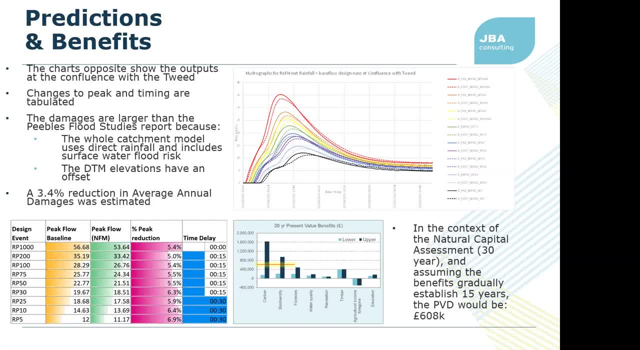 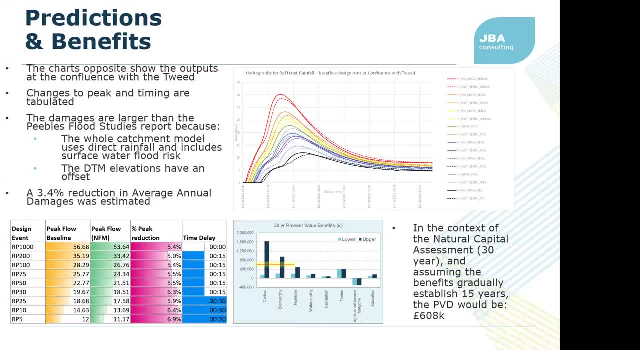 working at higher and higher events, then the integral of the damages across all those probabilities is going to be significant. so if it's used in combination with traditional risk reduction methods, then it's a useful thing to do. so you can also see one or two other things in there. 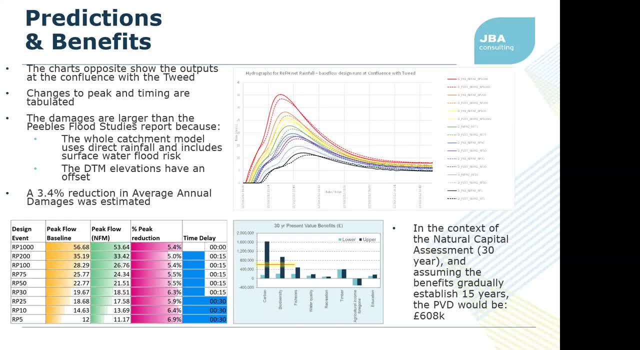 we've got the fact that the blue histogram, if you like, in the table, you can see that for very big events there's there's not much of a change in the timing, whereas there is with a small one. so there's a slight difference there and perhaps we might expect that too. so I'll go down to the next. 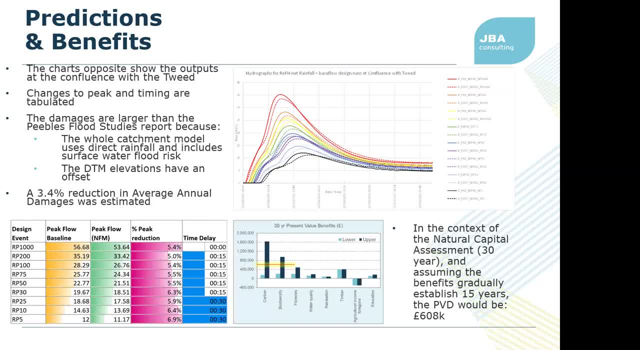 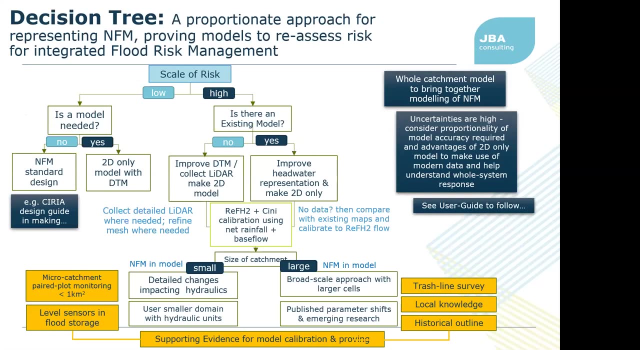 slide. so, having done all of those calculations and crammed them into that slide, we wanted to expand a bit on what we've done and how we've done it and also provide some sort of user guidance. so at the moment that's being produced and it will synthesize what we've written about a sort of decision tree. 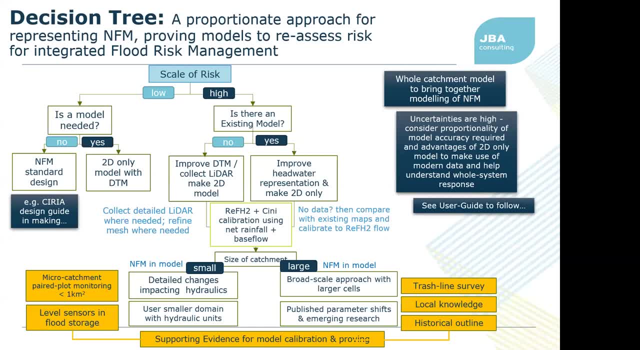 based approach for some of the things that I've summarized earlier on. so we've got. we want a proportionate approach for representing NFM, proving models, and when we want to reassert us flood risk or appraise flood risk and involve NFM, then why not be a bit more pragmatic and use? 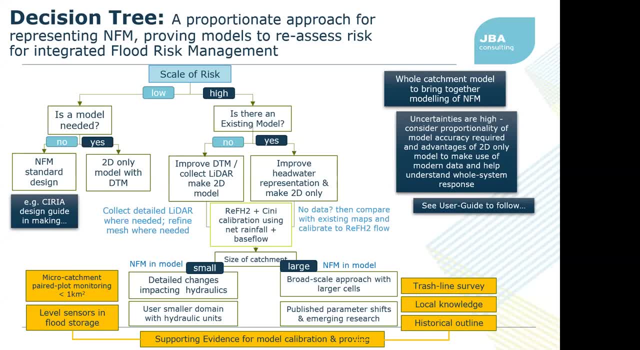 this kind of approach, depending on the scale of the risk. so you might even ask yourself: well, starting with the decision tree, is the? is the risk quite low? is a model actually needed at all? and we're awaiting a sort of Syria design guide that could give you best practice for implementing the NFM and, you know, put in place no regrets. 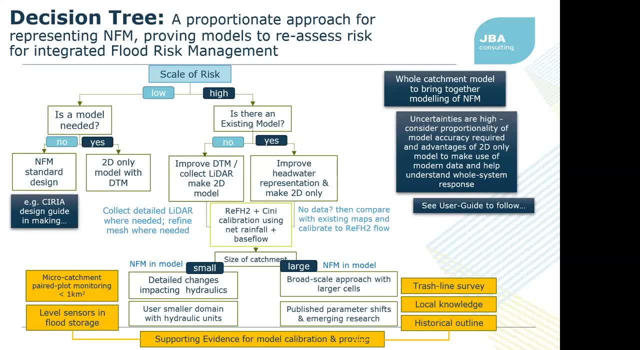 NFM to complement other measures, if there are any. but if that risk is a bit higher, then you might ask yourself: is there an existing model? and in Eddleston I've water. I've not really touched on phase one and how we incorporated earlier models. I can do that. there are. 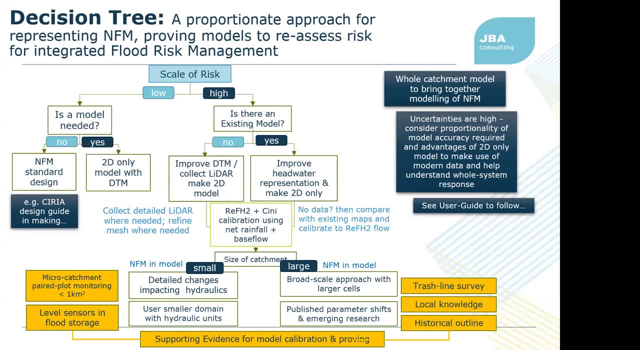 report outlines which models we've been able to sort of use information from and and, and. that has largely, in this case, been through using meshes that have been generated for parts of where an NFM has been implemented and bringing that into the DTM. so is there a model? no, well, perhaps it's. 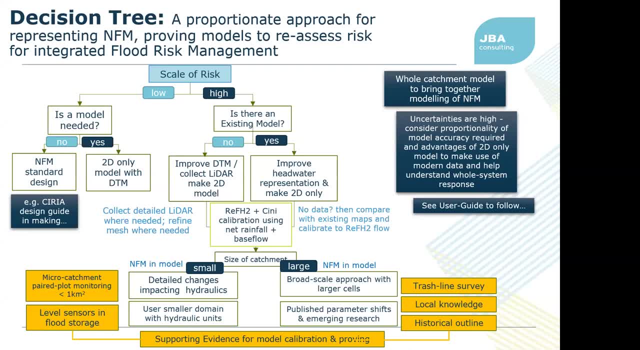 worth with the cost of lidar at this high resolution, coming down, collecting that and improving it and building a bit of a similar approach that we've just seen. if there is a model, and- and why not improve the head water representation, perhaps make it 2d. only you can have 2d flow areas flowing. 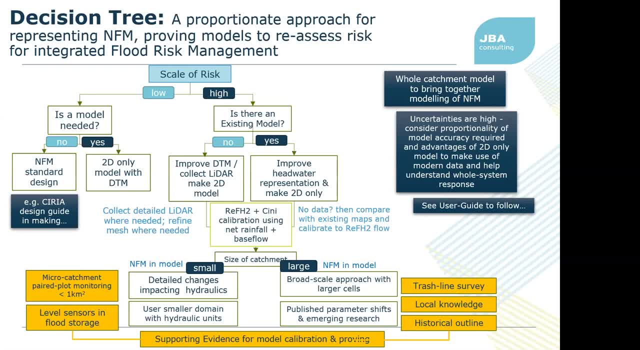 directly into a 1d or 1d 2d link model and in different packages. and then if you don't have any data- and we've done this in other catchments and you and there's no money to collect that data- then it's down to sort of trash line surveys and comparing with existing maps. for 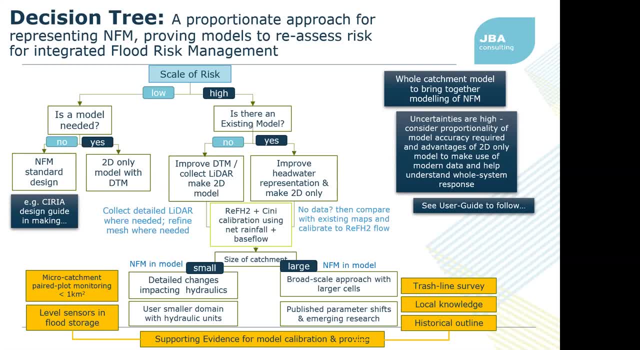 maps and also, and perhaps also the design hydrographs. so and, and, then we come down to: well, I think this is where I explained fairly succinctly in terms of: well, if it's, if it's small, then we could represent those detailed changes: hydraulic units directly in the mesh, refining the mesh, reducing the time step, and and. 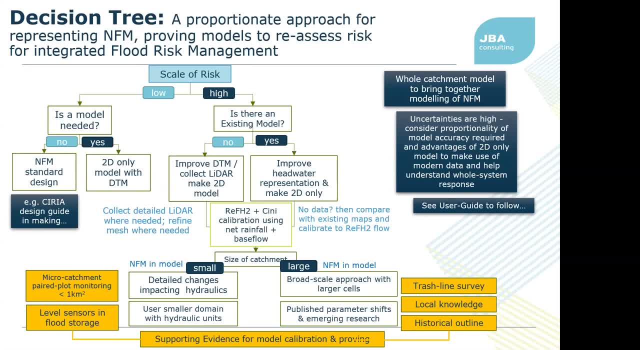 and. but we have to bear in mind that for for a small scale model that goes into that detail, you may want to have level sensors either side of every single unit in order to be confident in your coefficients that we mentioned, so that that might be better done as a demonstrator. 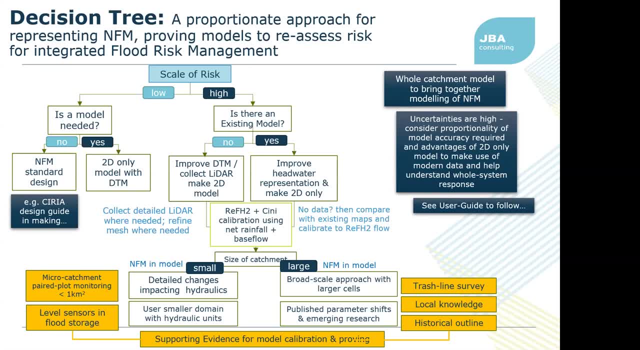 and that doesn't really come out in the decision tree. that well, um, but perhaps um in in a large catchment. just modeling and monitoring a portion of that catchment as a demonstration to show how it's working and then how it people can visualize how it will scale up at the large scale? yeah, we. 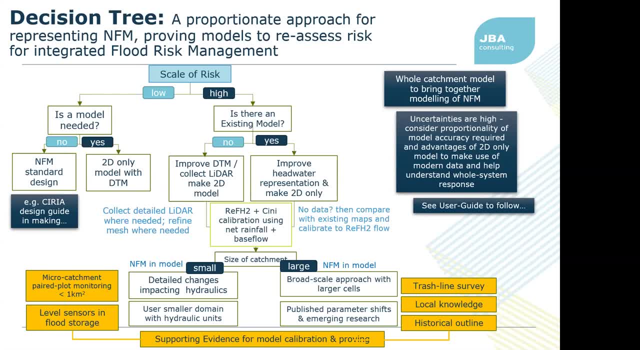 can use a broad scale approach with larger cells. we can use published parameter shifts and there's some nice literature there. now that's starting to summarize that and notably that Addy paper and some of the work coming out of the NERC projects. um, and you know, we should use whatever data we we can get our hands on in terms of understanding and 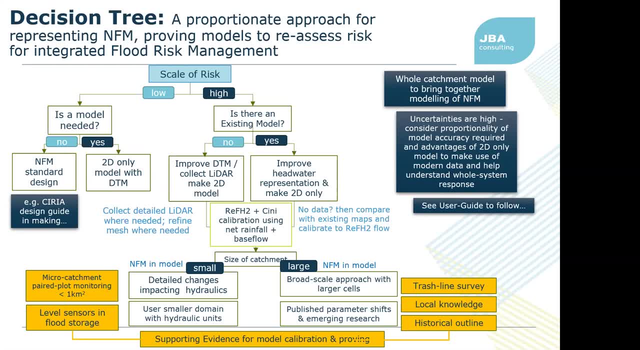 gaining confidence in that model. um, so um in terms of um sort of generating that user guide and and and bringing that into ways that we're probably going to have a draft of that already in sort of May um, and hopefully that will provide some useful guidance. um, in terms of um other, obviously there's there's other more fully. 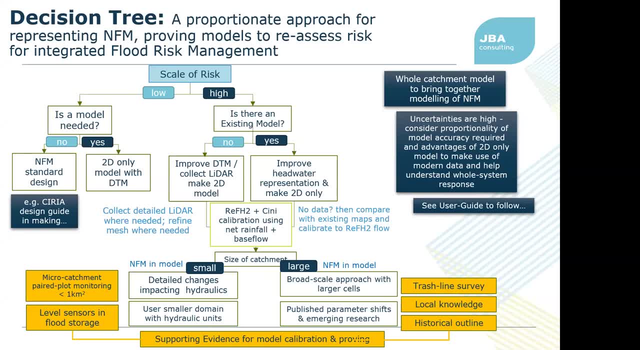 integrated modeling approaches which could be slotted in there if there's time and the modeling scale available, so you could use higher integrated models that include hydrology, um and and overland flows and so on, and some of the techniques that we've been um putting forward and publishing on uh. 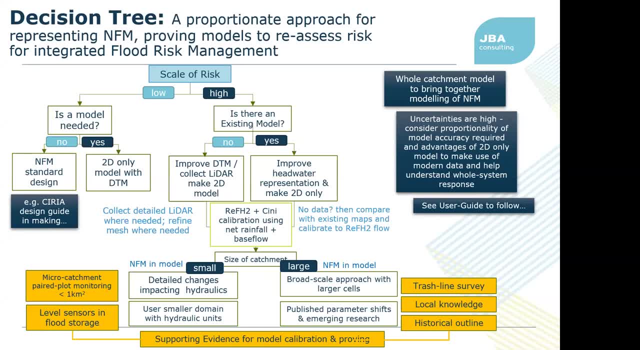 in QNFM have been things like: uh, taking the inputs from a distributed hydrological rainfall runoff model like dynamic top model, and inputting those into the channel network, in inputting the estimated runoff and through time to continuous simulation and then using a 2D hydrodynamic model such as 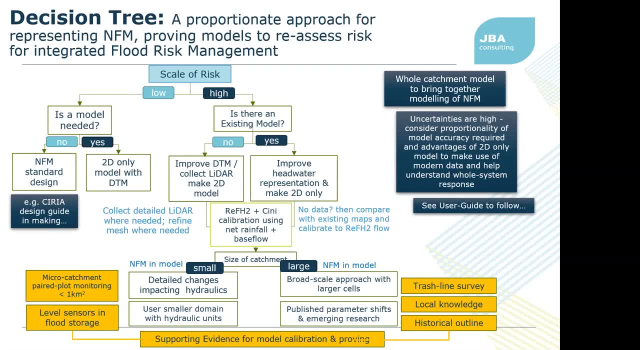 HECRAS or Gflow, and understanding hydrodynamics better around features like the ones we've been talking about. um, so, um, yeah, um, that that's where we've got to um with kind of uh, improving the learning from this study. um, obviously we we want to study the incentives a bit more and and that will provide. 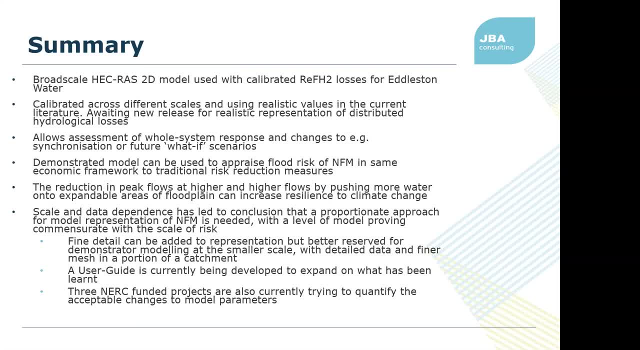 you with some, perhaps, ranges of values to what we've shown um. so. so, in summary, um, hopefully I'm not summarizing too early. I think it's 10, oh yeah, so I've been going 50 minutes. um, I think that the uncertainty analysis will show, you know, a bigger range and we can look at the. 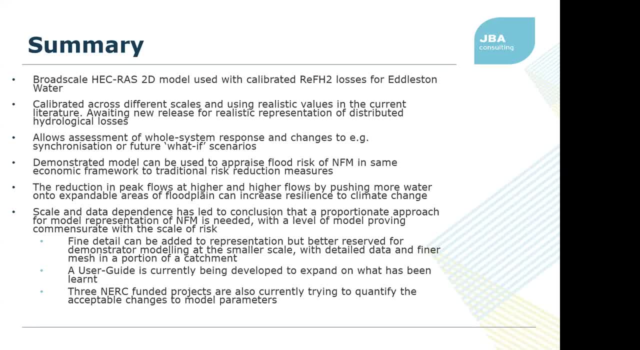 distribution of change. uh, with and without nfm. um, allowing for that parameter uncertainty, and we can look at whether that's significant as well. um, it does illustrate how difficult it is to detect change when nfm is causing some changes. but you've got that underlying environmental variability, so you're trying to detect something. 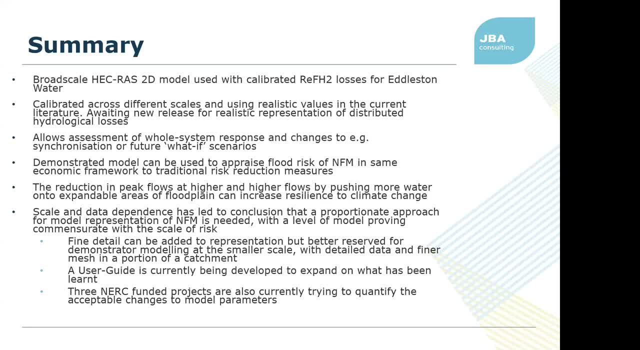 which is perhaps a smaller shift than the uncertainty in the observations as well. um, and it has been sort of calibrated across: um, the, the different scales and using realistic values of reference from the literature and the and the current um set of literature, um and um. we think it will probably improve a bit further. 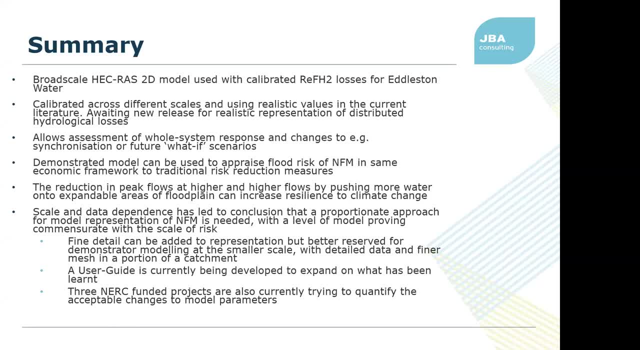 when we can have that distributed representation of hydrological losses, which should be in the next release, and then we could supplement the guidance based on that um. but that's something that would it that has been undertaken in other modeling packages. um, and for the reasons I've explained, we were going with hecarism. we've got faith that it has. 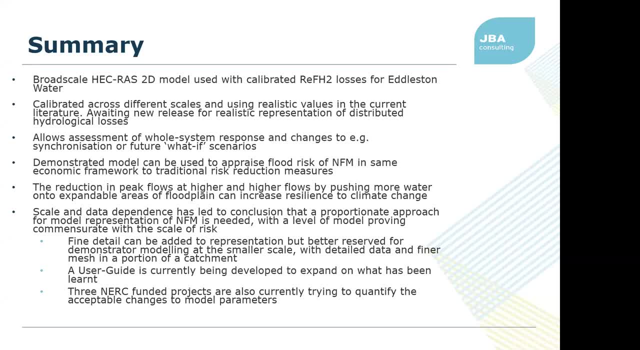 it's got some other important properties, um, and I think, um I, I think that it does give you um a system or an approach where you can understand: how is that- 70 kilometers squared um catchment, pushing water around? how is it interacting um, what are the kind of volumes being pushed around and and how has the 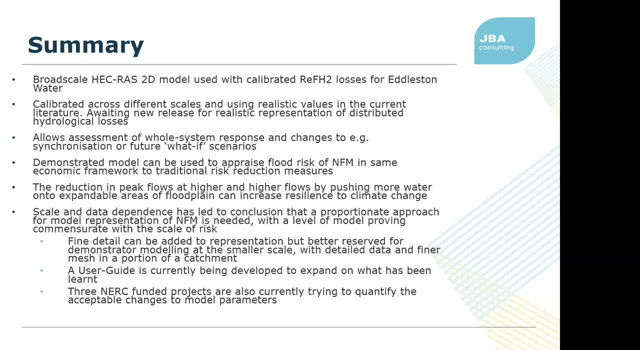 hydraulics been influenced and it might be that, um, you know, you could say that, within the uncertainty, the amount of water we're pushing onto the floodplain isn't hugely significant, but nonetheless, you've seen that, if that carries on like bigger and bigger events and we design our nfm right, so 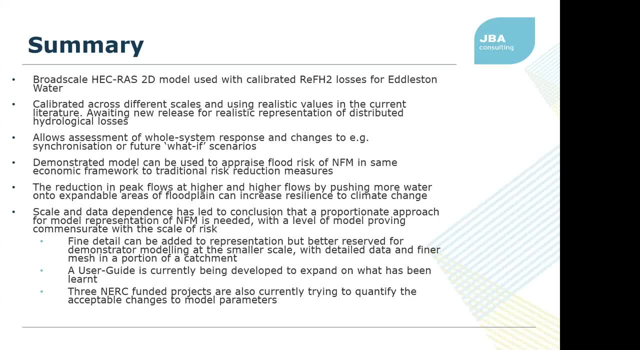 that it it accesses those pathways to more expandable storage, then it's nfm is playing a a useful role in making catchments more resilient to climate change. so, um, in terms of um, uh, different studies having probably much less data than this, we've tried to make a flexible kind of approach to incorporating nfm within a study and we've shown 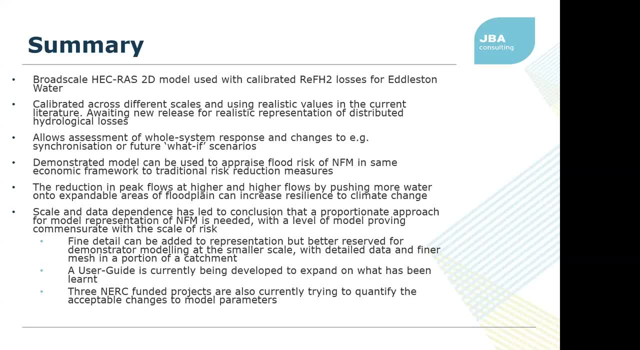 might appraise the risk based on that, With the level of model proving that's commensurate with the scale of the risk. So we can't build this model. there's not often enough funding to take a cross sectional survey of a catchment this size if it's not been already build. 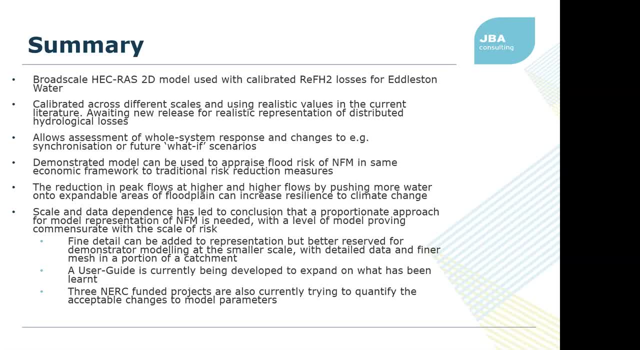 a 1D, 2D link model. We're talking an awful lot more money than was spent building this demonstrator model. But what we can do, we can represent the fine detail in a portion of the catchment. we can demonstrate how it's working. we can have a bit more confidence. 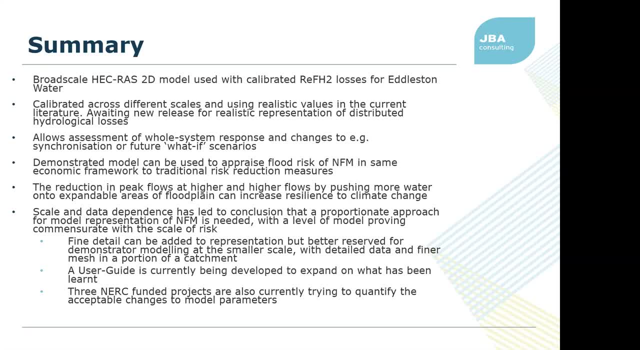 and then we can say, well, if we do this in the rest of the catchment, like we've done with the model, so those engineered log jams on Middleburn were calibrated and then we've had trust that they're working because we've got a reasonable fit with the post-NFM piece. 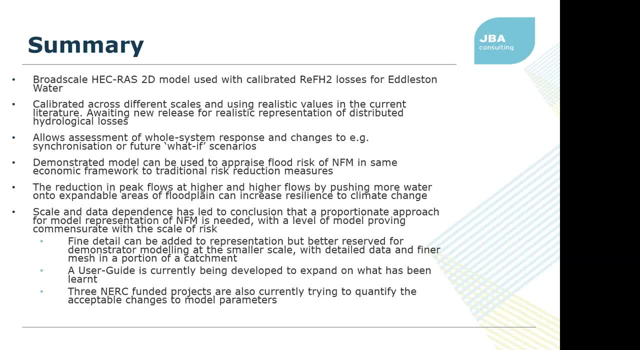 of peaks And so we've used the same values elsewhere in other sub-catchments, Then it's a similar phenomenon. really, if you can show things at a small scale and show how they might work at a larger scale, And also bearing in mind that you can use this type of approach, 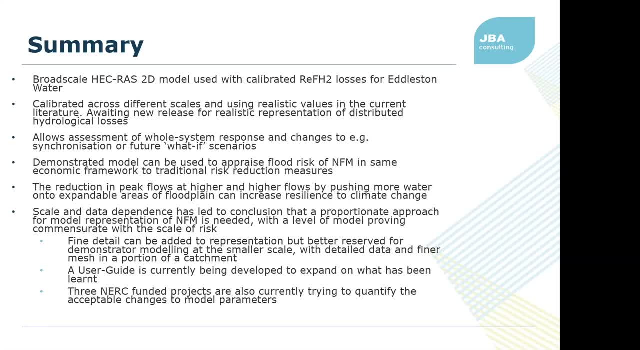 to understand the synchronisation of peaks and perhaps just slow down those slower rising peaks, Rather than trying to slow down the faster rising ones which might get ahead of the main flood peaks. So it does enable you to do that kind of what-if scenario. The user. 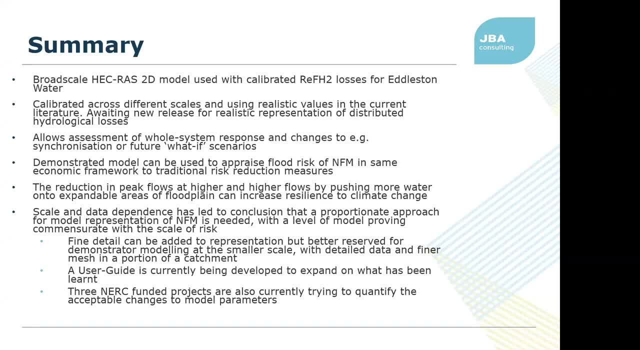 guide's not quite finished yet and we'll hope to get that out soon, And I think it would be wise to follow the progress of the three NERC funded projects which are also commenting in all these areas. But it's been really nice. 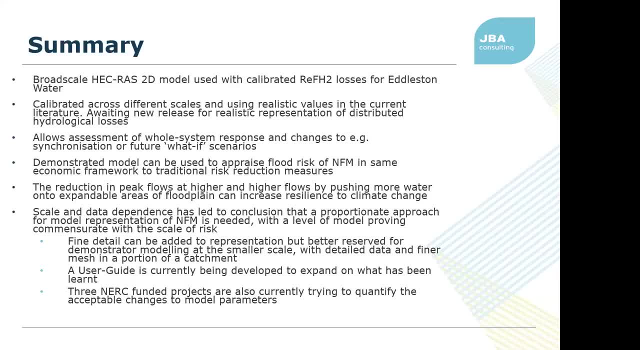 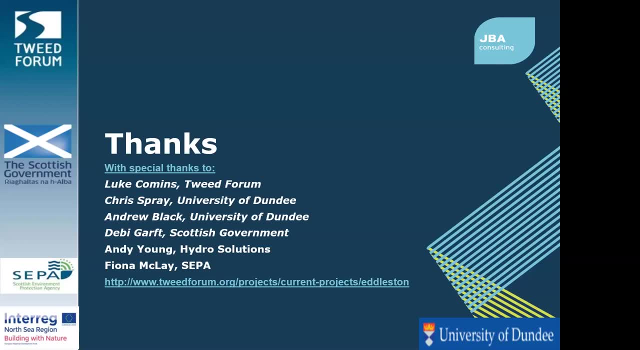 It's been really nice to work with the partners with their really detailed set of monitoring data, And I know an awful lot of hard work has gone into collecting that data There's been- there hadn't been at the time of writing, if you like- a very big post-NFM event And 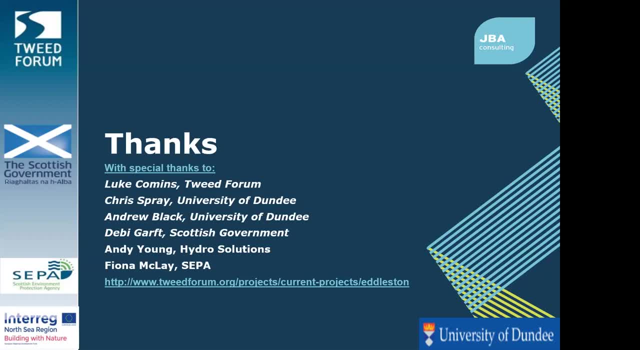 I look forward to hopefully being involved with looking at how that could be modelled now that there are some Thank you. I know that those bigger events will improve the ratings And because I'm not having enough large scale flow ratings to improve those telemetry- sorry, the gauging- And once that's. 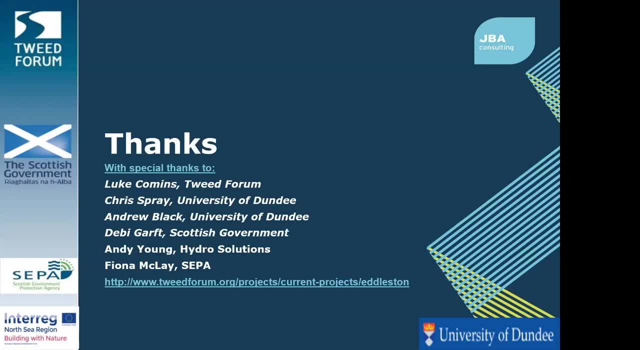 in place, we would reduce the uncertainty in the return periods which I showed between RefH and the statistical method. So we'd hope eventually to use the Kitson-Mill gauge to improve those design hydrology. So with that I'll leave you with the link to the Tweed Forum's Edelston project And 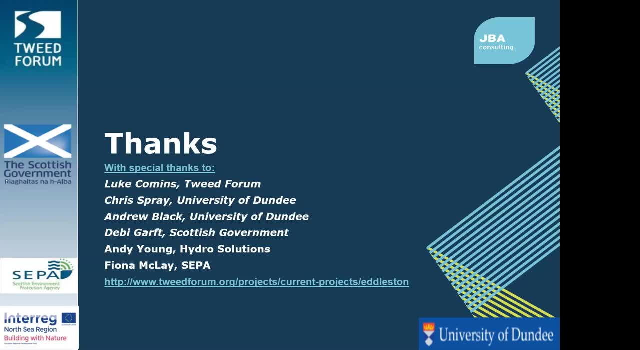 I think there's some time for questions. Thank you very much, Barry. Really interesting comprehensive presentation. We have. Zoom really needs a digital applause button, doesn't it really? It's not quite the same when you're doing it here. 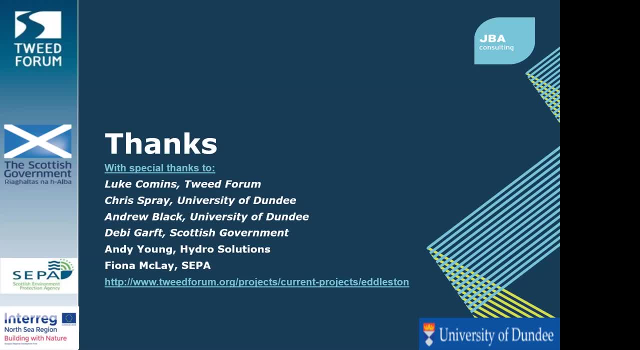 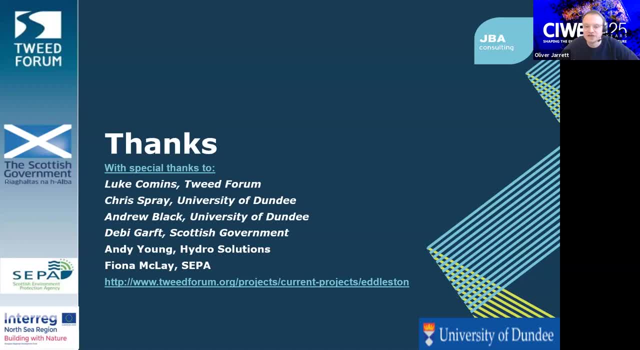 Yeah, Yeah, Yeah, Yeah, Yeah, Yeah, Yeah. Very good, Great. you presented some maps with an urban area. Isn't that much more likely to be incorrect using a 2D surface flow model, given urban structures and local drainage systems? 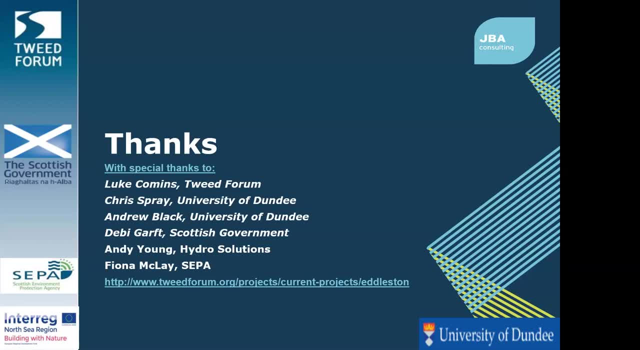 Yes, I'd agree with that. We are trying to model NFM. We went in the business of modeling suds and so on, although they can have a big effect. As soon as the new functionality is available in HECRAS, we'd be able to alter the local net rainfall having a drainage factor much like in. 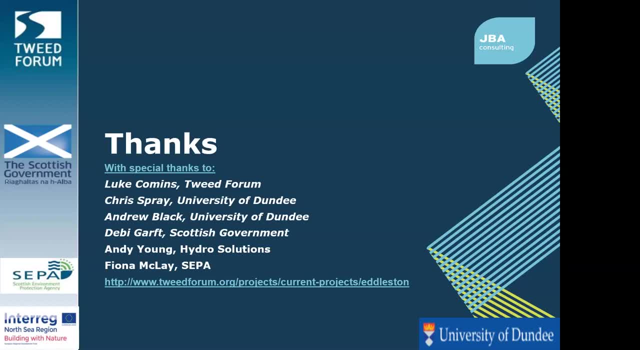 the surface water map generation. We weren't trying to do that in this study. Paul Webster says: hi, Barry, many thanks for the presentation. I was surprised at the consistent reduction in flow peaks across all return periods. I was expecting there to be a reduction for higher. 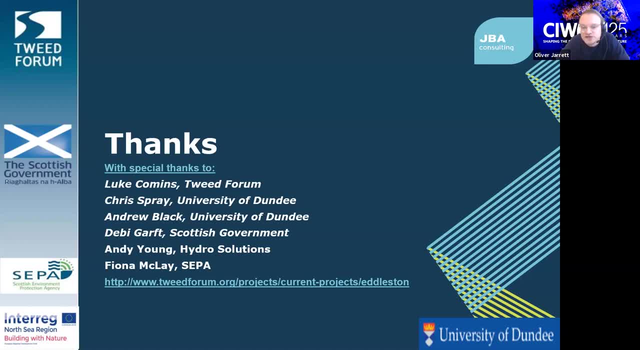 return periods. I was expecting there to be a reduction for higher return periods. Have you any thoughts on this? eg, is this due mostly to the increased flood storage volume? Well, I think in this instance, some of these NFM features have been designed quite well, You saw. 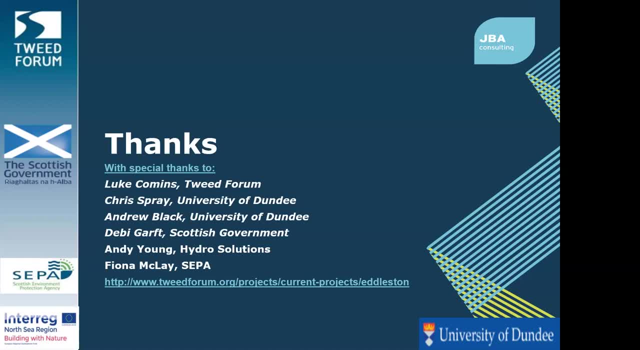 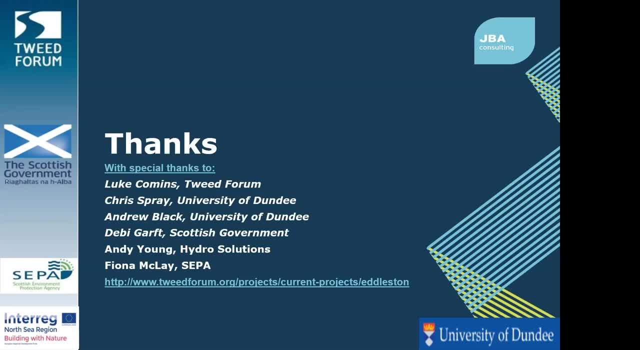 I would have from the Datsun type paper. you'd expect a lower return period, So I suppose it is slightly surprising. It could be a facet of the modelling we haven't yet uncovered. but when I look into details I typically find in quite a lot of areas in riparian land where we've 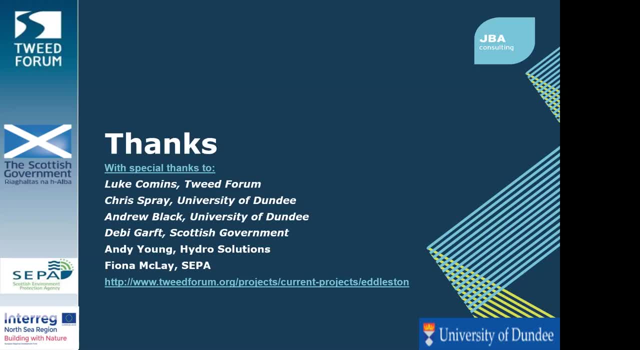 promoted more connectivity with the floodplain. I would have from the Datsun type paper you'd expect plane more water is being pushed there. So you can see- and I've got some more sort of evidence for that from other studies- we can see more and more. we could see it in a couple 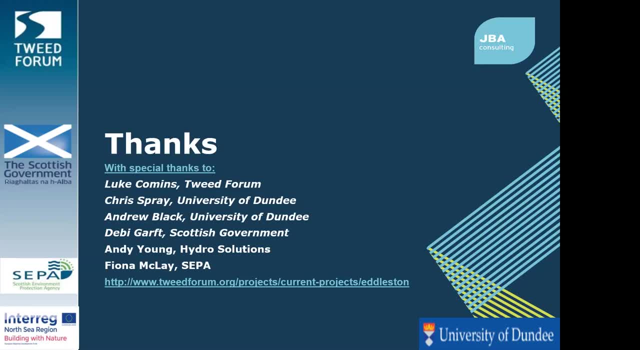 of those plots I showed more and more storage as the flows get bigger. Okay, Patrick Taylor asks what is the reason for not using 1D modelling and purely 2D And, generally, which NFM measures were used for this study catchment. 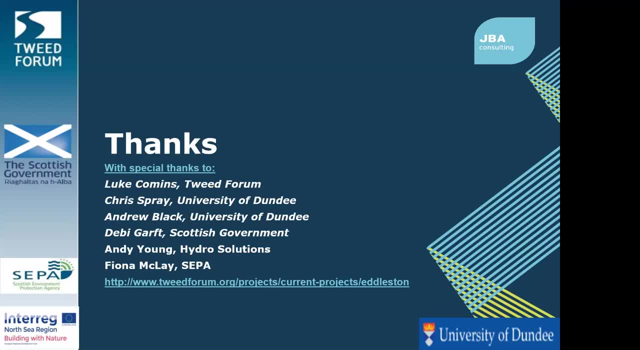 Okay. Well, I guess if you're going to use, if you've got all this wonderful 2D information that's more and more available from SEPA and Environment Agency and other partners, then you're going to get a better picture of the truth, of what the topography is doing than 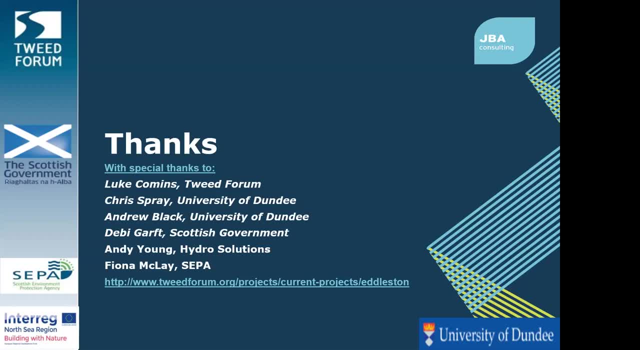 an interpolation between 1D cross-sections and using panel roughness and so on. I think the future of this kind of 2D modelling is going to be a little bit different. I think the future of this kind of whole catchment modelling really is to understand how the 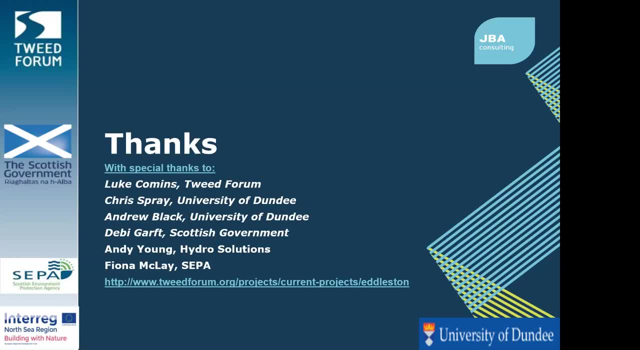 different flow accumulation pathways are interacting continuously. The model presented, really, you can only look at design events and sort of single peaked events. It would be difficult to do continuously. So and in terms of the NFM represented, I think I sort of outlined. 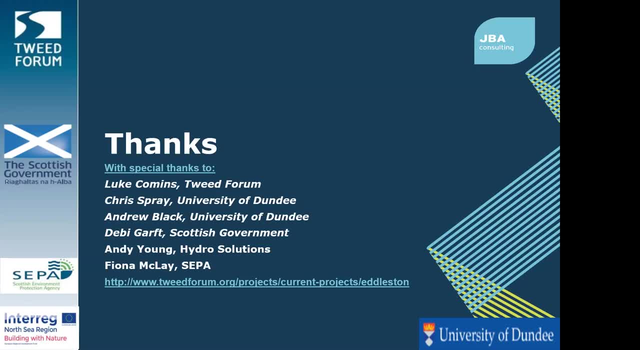 that, in terms of it, was things In terms of woodland, in terms of hydraulic structures and so on. We did do some other scenarios that haven't been presented here in terms of representing improvements to soil structure, just purely by increasing the soil storage. We did that as a sort of global change. 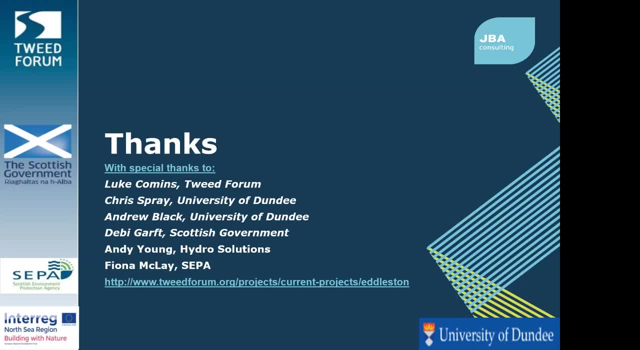 We've often done that as a as a percentage change to distributed hydrological parameters. Okay, And so in the models that you've seen, we haven't been doing that for the tree planting, but it's something else that should be represented in the future. They, of course, have woodland. 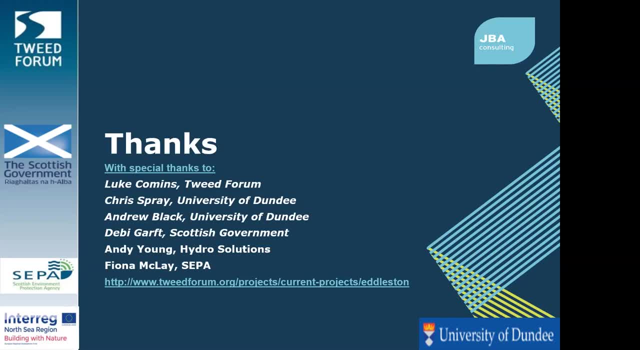 will have an effect on friction, It'll have an effect on increasing infiltration rates and it'll have effect on wet canopy evaporation rates. Okay, And we'll probably finish here with one, that where we step away from the modelling detail for a bit. 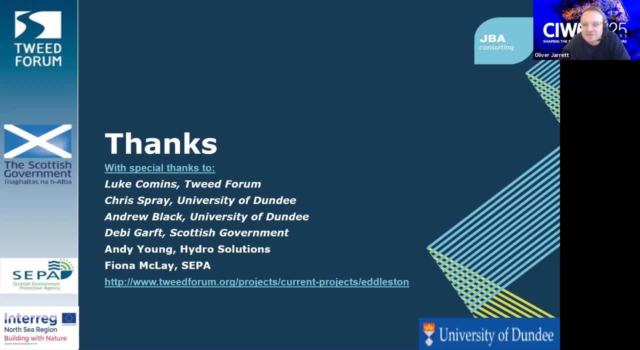 And Ashling asks: what has the response to the project been like from community or land owners and or landowners? I think I think the person to answer that would be probably won't be able to talk on Zoom right now, but I think Luke would probably be able to give the best response to that. 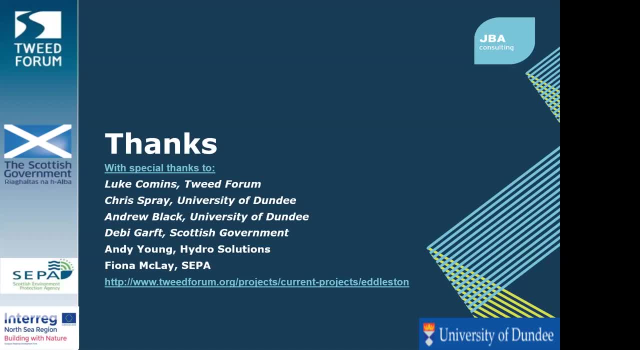 It might be that that's one where we can have a kind of written response, but I understand that it's been well received, Okay, And that I also understand from Chris that there's been quite a lot of educational events in schools and so on where it is well received. 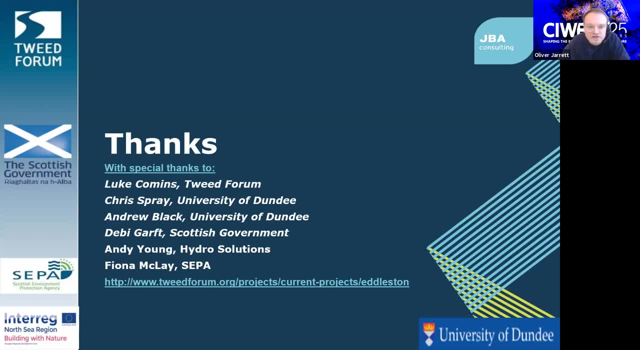 Okay And we'll do another one quickly. that's kind of linked into that. David Bassett asks how important are larger land use changes and naturalisation as opposed to localised NFM features? Nice question. That's something that I wanted to actually point out. was you know there? 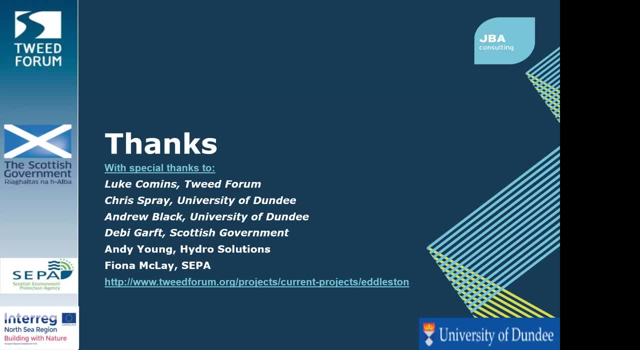 does need a lot of NFM has been quite small scale. There's a growing amount of it, But I think we do need to be ambitious about how much of the riparian land is used, And I think that goes into the whole payment for public goods arguments. So I think if we're thinking 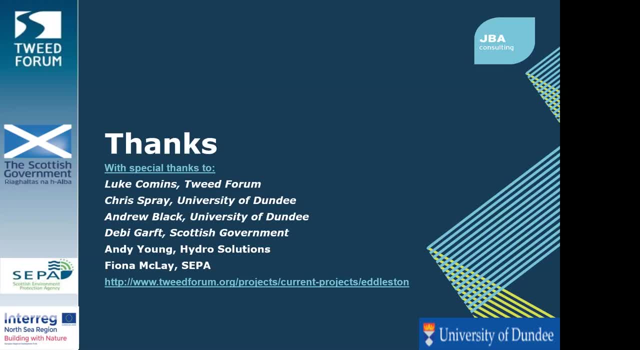